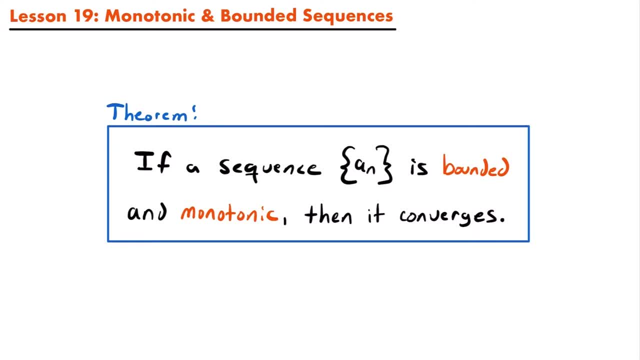 towards by the end of this video. What this specific theorem tells us is that if a sequence, a sub n, is bounded and monotonic, then it will converge Alright. and so at the end of this video, we're going to circle back to this theorem and try to determine the convergence of some. 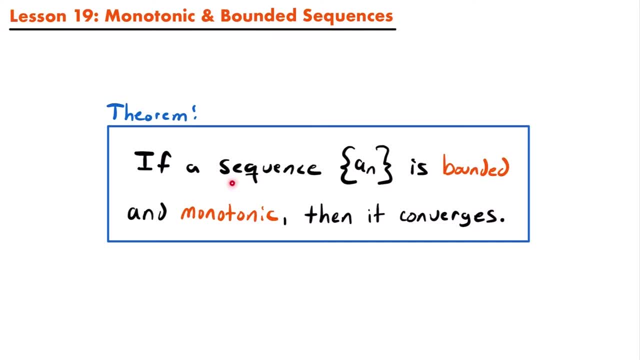 sequences, But first we need to establish what it means for a sequence to be bounded and for a sequence to be monotonic. And we're going to start by looking at the convergence of a sequence without using a limit. And we're going to start by looking at 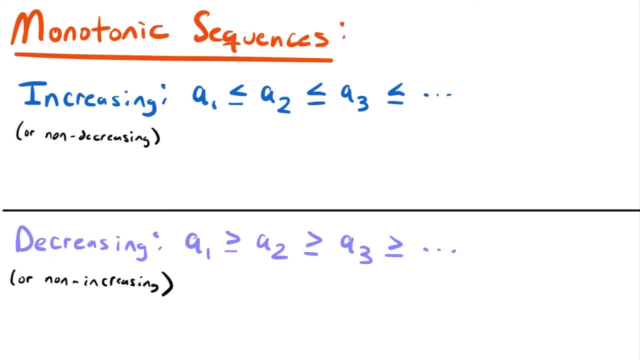 what it means for a sequence to be monotonic. Alright. so monotonic sequences are sequences where the terms either increase or decrease with each subsequent term, And so a monotonic sequence that is increasing the first term will be less than or equal to the second term, which will be 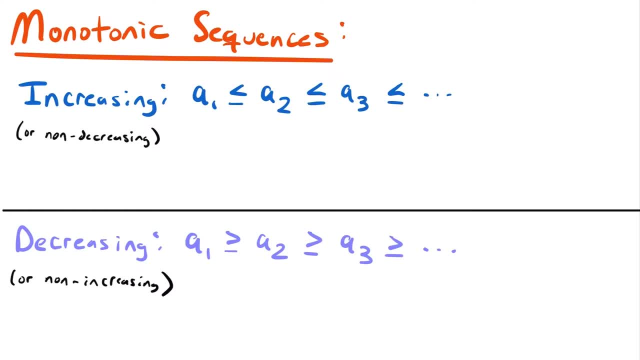 less than or equal to the third term, and so on, And sometimes you'll see this called non-decreasing instead of increasing. That's just because there is a possibility that your terms would be equal to each other, and so on and so forth, And sometimes you'll see this called non-decreasing instead of. 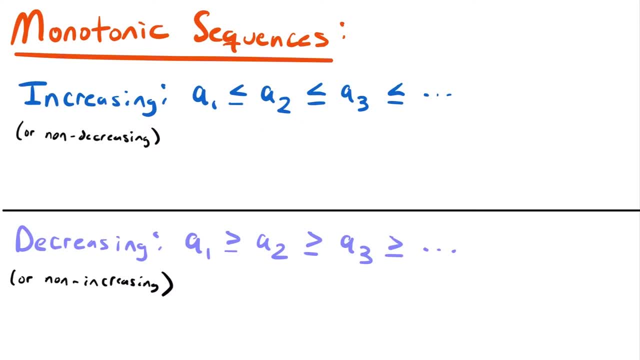 increasing. That's just because there is a possibility that your terms would be equal to each other rather than being less than the next term. However, that's not going to occur a lot, and so it's easier just to say that the terms are increasing rather than non-decreasing. 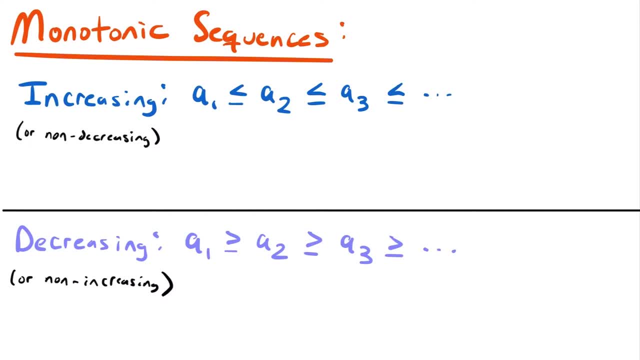 Alright, so, in a general sense, what we can say is that, for the nth term, a sub n that is going to be less than or equal to the next term, which will be a sub n plus one. And so when you want to show that a sequence is increasing, which would make it monotonic, 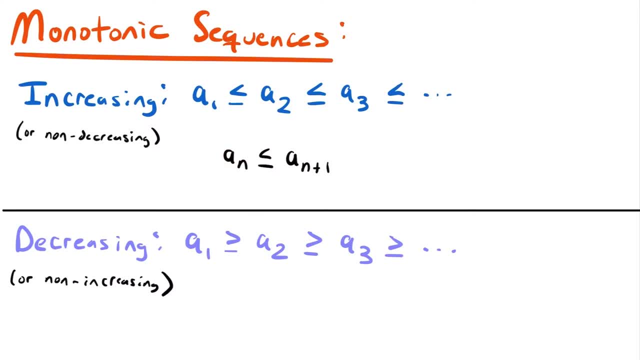 you would want to show that this statement is true, that a sub n or the nth term of the sequence would be less than or equal to the n plus one term for that sequence, And if you were to divide both sides by a sub n plus one, another way you could express this. 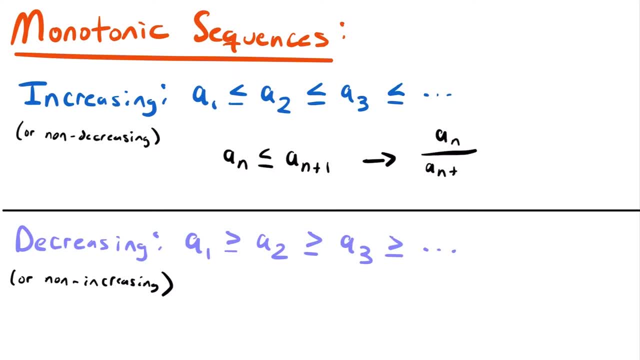 is that a sub n divided by a sub n plus one would be less than or equal to one. So that's an alternative way to express that A term of your sequence divided by the next term of your sequence should be less than or equal to one. Now, if your sequence is decreasing, 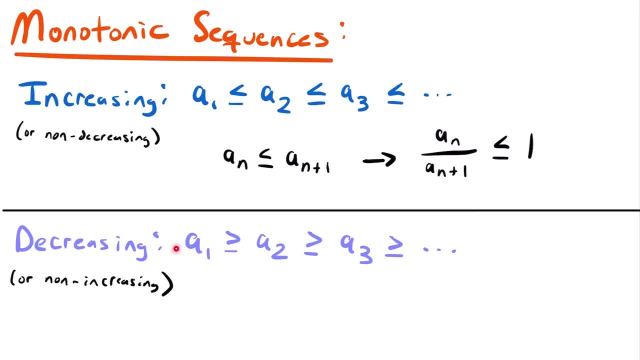 that's another way that it could be used to show that the sequence is decreasing. That means that each subsequent term of the sequence is less than the previous one, and so your first term, a sub one, would be greater than or equal to your second term. 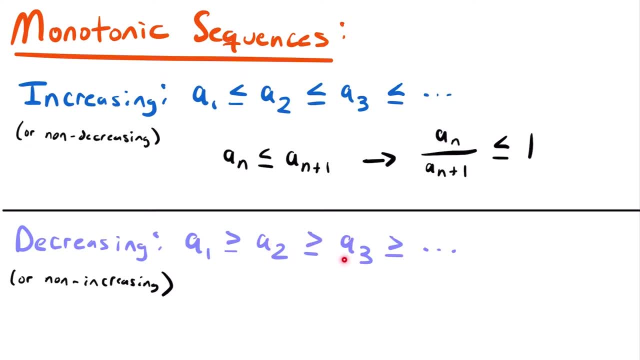 your second term would be greater than or equal to your third term, and that would be greater than or equal to your fourth term, and so on. Now, once again, just like how we call increasing non-decreasing, because the terms could be equal, the terms could also be equal here. 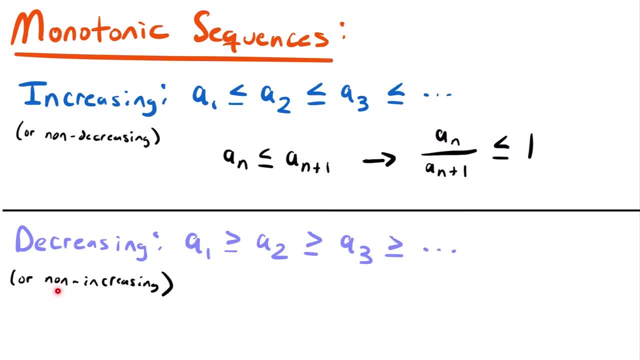 in a decreasing sequence, and so you might see this called non-increasing And so, similar to what we did up here. in general we would say that a term, a sub n, would be greater than or equal to the next term, a sub n plus one right. So for an increasing sequence, a sub n will be less than or. 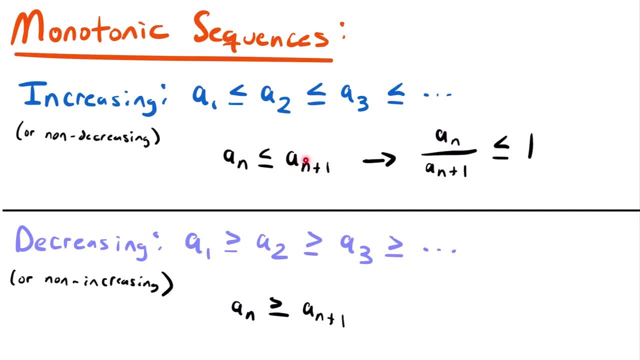 equal to the next term. That term is greater than the previous term, so that's why it's increasing. But for a decreasing sequence, the next term after a sub n is going to be less than that previous term, and so each term gets smaller and smaller, which means that the sequence is decreasing. 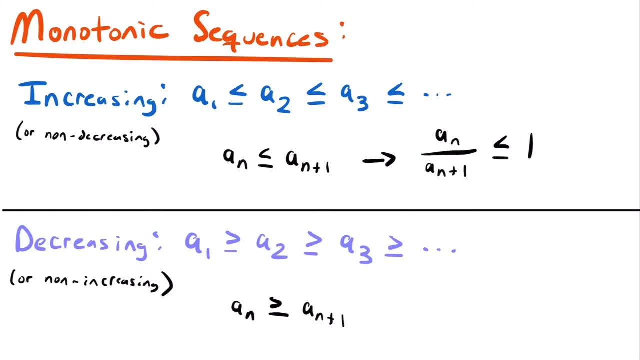 And then, similar to what we did up here, for an increasing sequence, if we divide both sides by a sub n plus one, you can see that if a sub n divided by a sub n plus one is greater than or equal to one, then that means that your sequence is decreasing. And so you could. 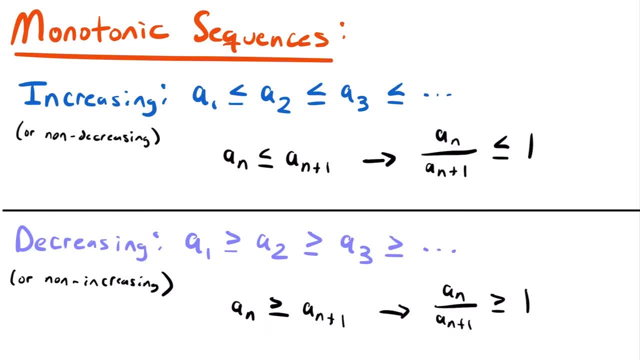 use either of these statements to show that a sequence is increasing or decreasing, which would mean that it is monotonic, And we will be looking at examples of using this definition to show that and show you visually what a monotonic sequence looks like and what a sequence that is not. 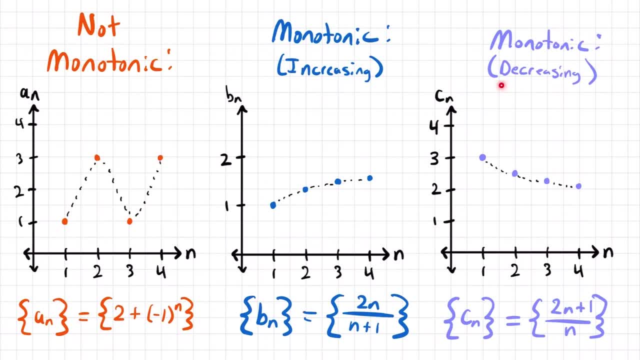 monotonic looks like as well. All right, so here we have three graphs to take a look at. Each of these graphs is a representation of the terms for the sequence below it, and for each one of these graphs, the horizontal axis represents our values of n. 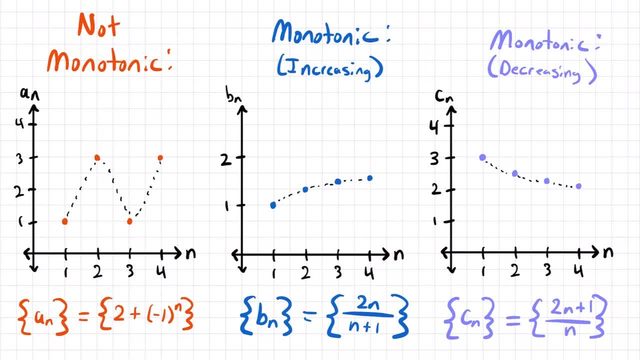 and the vertical axis represents the value of the term at that value of n. And so if you take a look at our first graph here, this represents this sequence: two plus negative one to the past power of n. and if you look at the graph, when n equals 1, our term is 1, when n 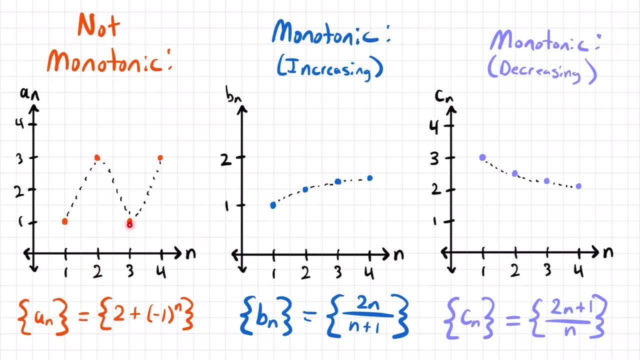 equals 2, our term will be 3, and then we go back to 1 when n equals 3, and then back to 3 when n equals 4.. And so this sequence oscillates between 1 and 3 for its terms, and so there isn't a clear pattern that each subsequent term is. 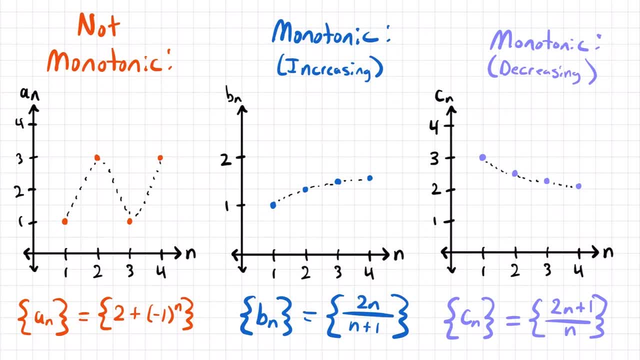 either getting larger or getting smaller. It can only go in one direction. In this case, it's going in both directions: We're increasing, then decreasing, then increasing, and then we'd be decreasing again if we were to continue on and then increasing, and that would continue forever, And so this sequence oscillates. 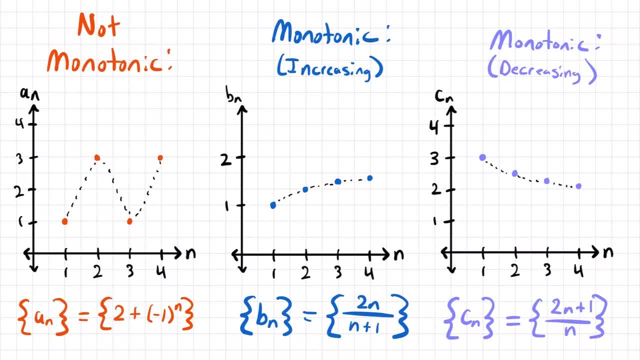 between two values, and so it's not monotonic. It is not headed in one direction, whether that be by increasing or decreasing. For our next graph, this is an example of a monotonic sequence that is increasing, and this is the sequence right here: 2n divided by n plus 1.. When n is equal to 1, our term is 1, when n. 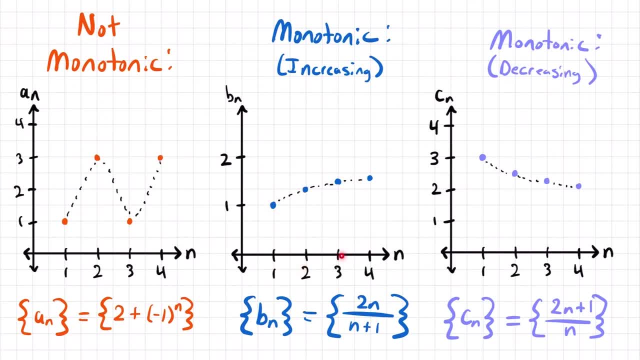 equals 2.. Then we're going to go back to the previous graph and we're going to go back to our previous graph. We're a little bit higher than 1.. When n equals 3, we're even higher above 1, and then at n equals 4, we are even higher, And so each subsequent term. 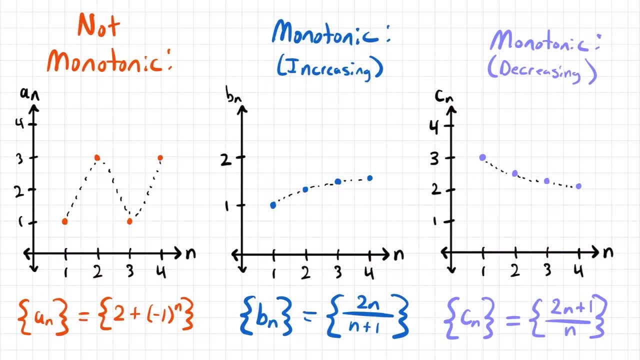 is getting greater than the previous term, And so, because each term gets greater, this is an increasing sequence, which means it's monotonic. And then for our last graph, this is an example of a monotonic sequence that is decreasing. Each subsequent term is going to be less than the previous term, and so this graph. 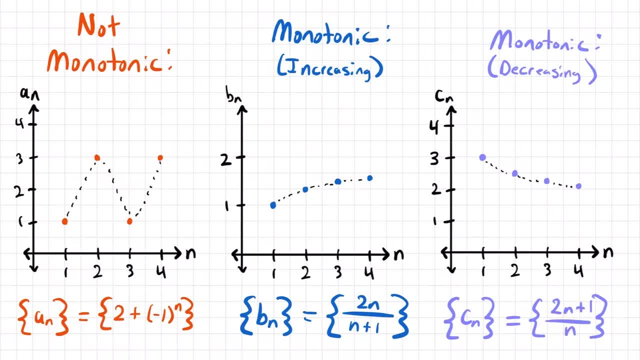 represents the sequence 2n plus 1 divided by n, And so at n equals 1, we have a term of 3, and then, at n equals 2, we have 2.5, and then, at n equals 3, we're even lower than 2.5, and then, at n equals 4, we 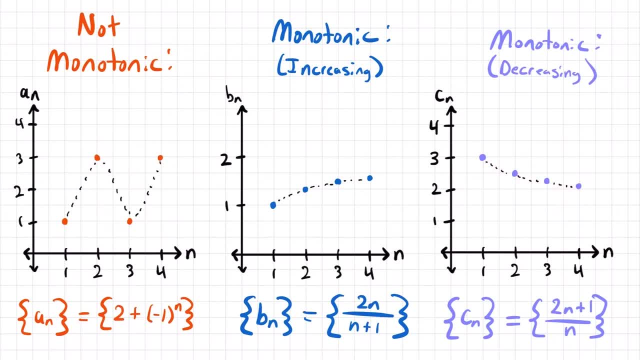 get even lower, And so each subsequent term is smaller than the previous term, and so this is a decreasing sequence, which means it is monotonic, Alright, so hopefully these graphs help you to visualize what exactly are monotonic sequences. What do they really look like when you graph their terms? But now we're ready to. 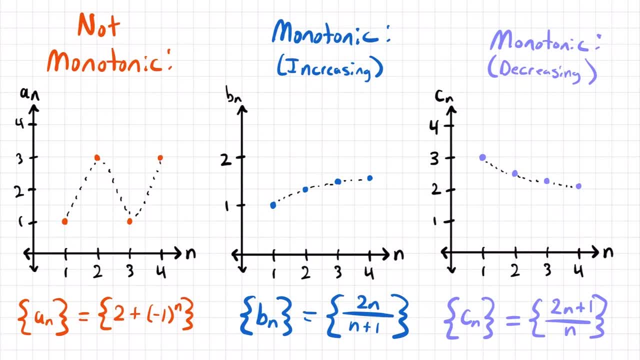 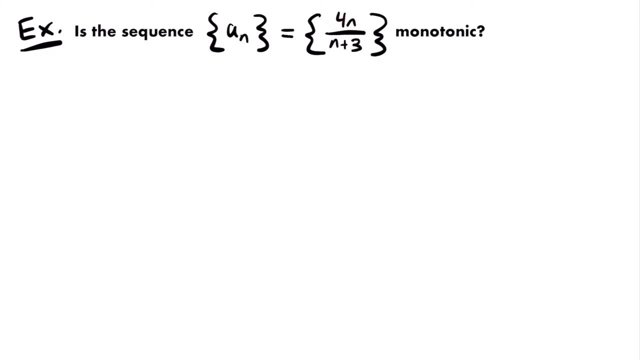 actually look at a sequence and determine if it's monotonic or not, And so here's our first example. We want to know: is the sequence- a sub n is equal to 4n divided by n plus 3- monotonic? And so here's how we're going to determine. 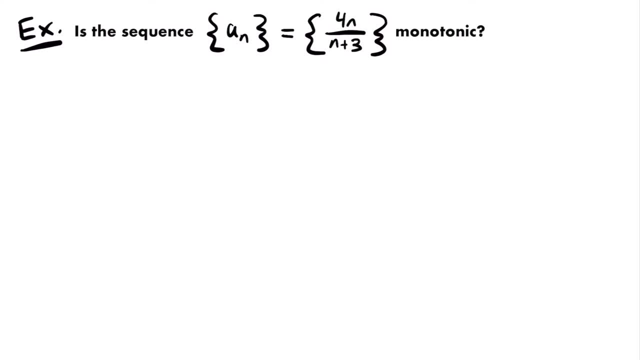 whether this sequence is monotonic or not. We're first going to list out some terms. Typically, I like to write out the first four terms. I think that gives us a good look at our sequence, And if we see that the terms are either increasing or decreasing, then we are going to try to 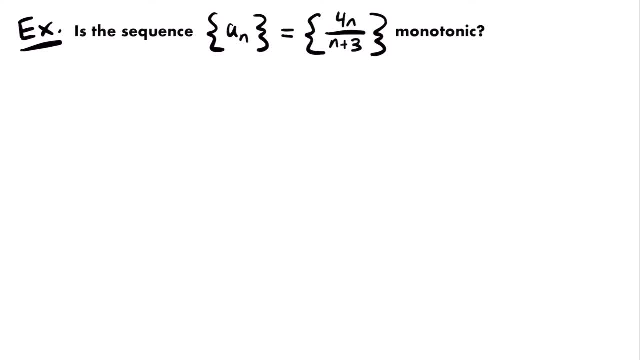 prove that by using one of our general statements from earlier for an increasing or decreasing sequence, And I'll show you what that looks like when we get there. but let's start by just writing out the first four terms of our sequence. So first we're going to have a sub 1 where n is equal to 1, and so that 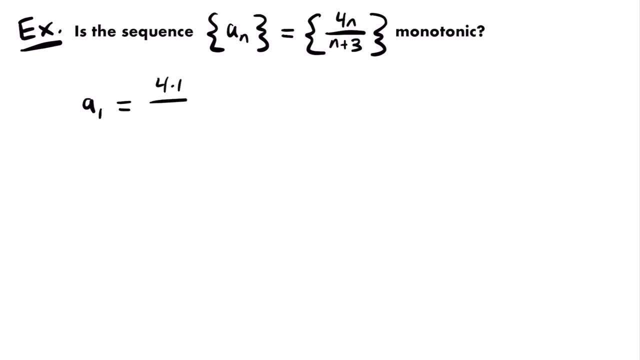 will be equal to 4 times 1 divided by 1 plus 3, and that will simplify to be 4 divided by 4.. and that's equal to 1.. Now let's work on a sub 2.. So a sub 2 will be equal to 4 times 2 divided by 2. 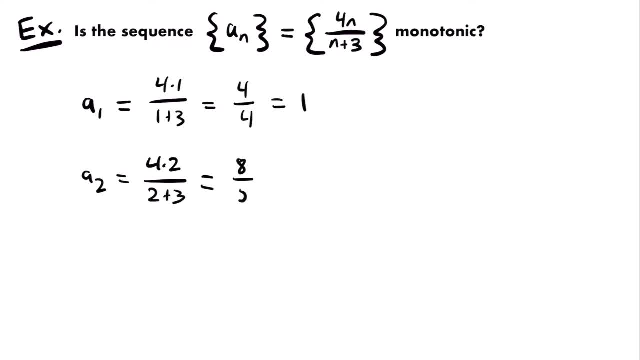 plus 3, and that will simplify to 8 fifths, and that in decimal form is 1.6.. Then a sub 3 is equal to 4 times 3 divided by 3 plus 3, and so that's equal to 12 sixths and that is equal to 2.. And 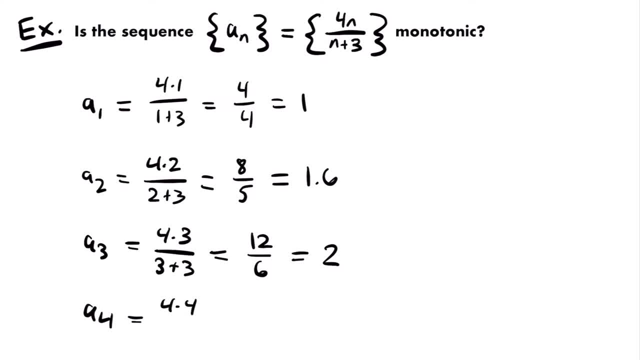 then for a sub 4, that will be equal to 4 times 4 divided by 4 plus 3, and that is equal to 16 divided by 7, and 16 sevenths is approximately equal to 2.29.. All right, so now for each. 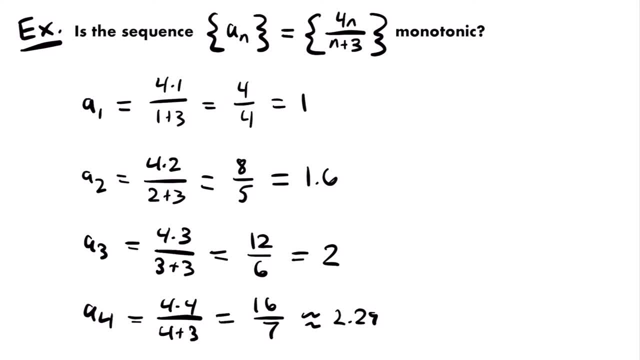 subsequent term. we can see that the next value is greater than the previous value. We started at 1, and we have 1.6,, which is greater than 1.. Then we have 2,, which is greater than 1.6,, and then we 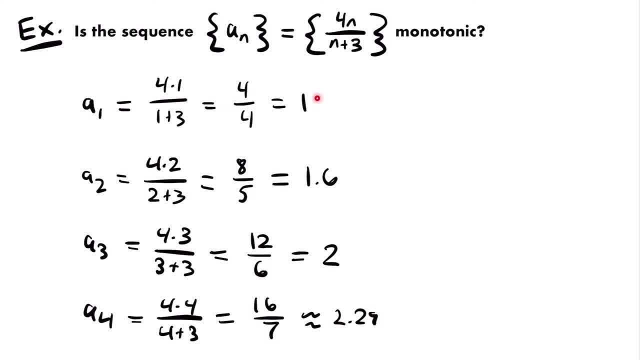 have 2.29,, which is greater than 2.. And so we can see that each term is getting greater. so we know that this sequence is increasing, but we need to prove that, We need to show that it's increasing so that we can conclude. 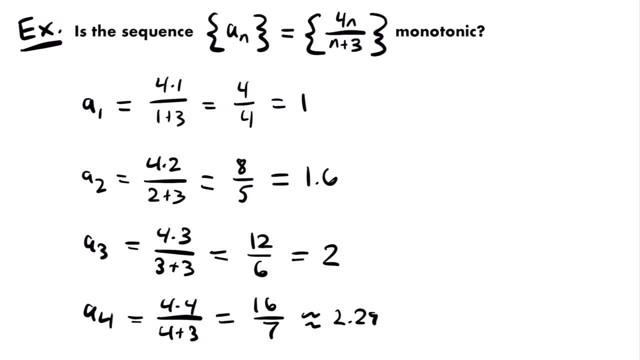 that it's monotonic, And so here's how we're going to do that. Remember that we said, for an increasing sequence, that the nth term, a sub n, will be less than or equal to the next term. a sub n plus 1, right, The next term will be greater than or equal to the previous term. 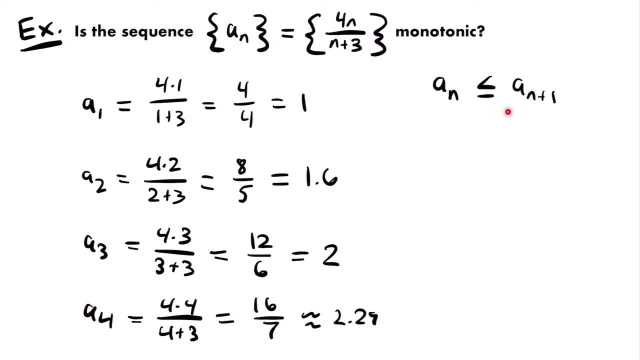 and that's what we found here, And so the way we will prove this is by replacing these terms with what those terms would look like for this sequence. So we know that a sub n will be 4n divided by n plus 3, so we'll have 4n. 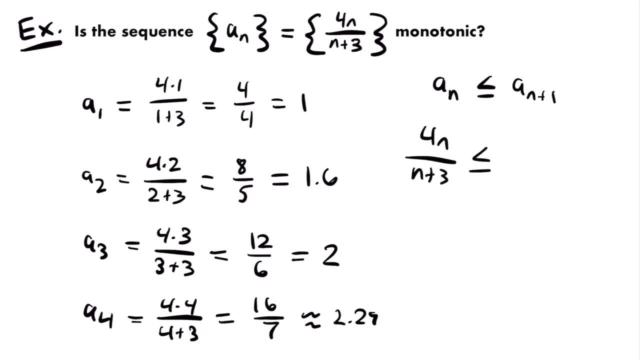 divided by n plus 3, and that's going to be less than or equal to a sub n plus 1.. So we're going to use that same sequence but replace n with n plus 1.. So we'll have 4 times n plus 1 divided by. 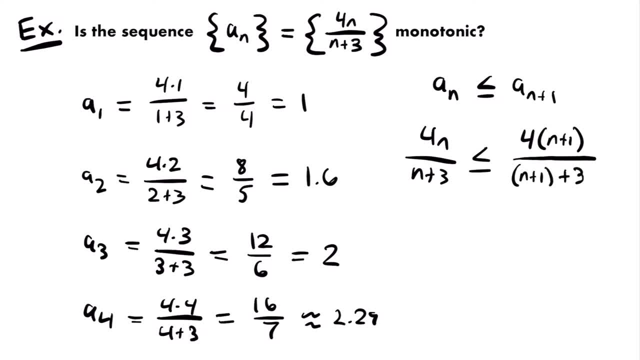 n plus 1 plus 1.. And that will come out to be equal to n plus 3, right? We just replaced each n in our sequence with n plus 1.. Now, if we simplify a little bit, we can distribute this 4 through this quantity. 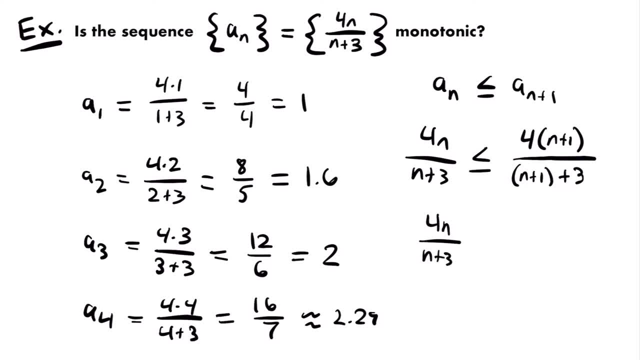 and then add 3 and 1.. So I'll have: 4n divided by n plus 3 is less than, or equal to, 4n plus 4 divided by n plus 4.. Alright, and so then, what we want to do is simplify this inequality as far as we can, up until a point where we can determine if that inequality is equal or one. 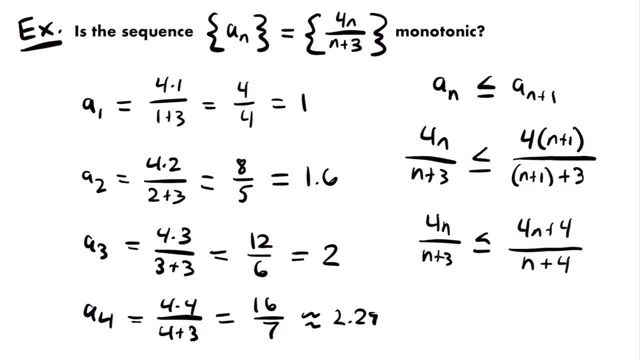 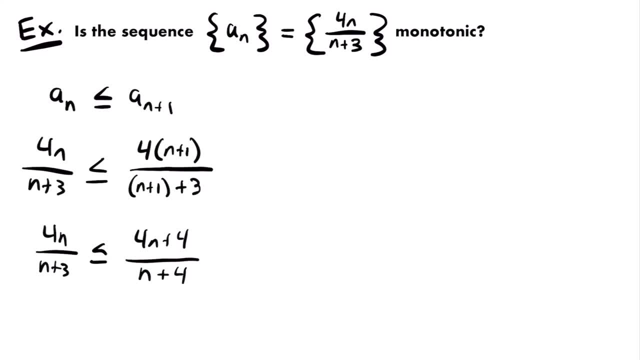 is true, And so what I'm going to do here is clean up my work, and then we're going to further simplify our inequality by cross multiplying. In other words, we're going to be multiplying both sides by n plus 4 and multiplying both sides by n plus 3 to cancel out those factors in the 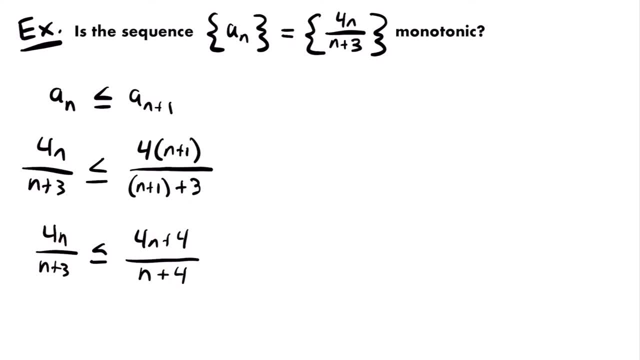 denominators. But an easy way to think about that is just to cross multiply. So 4n times n plus 4 is going to be on this side of the equation. So we have 4n times n plus 4 and that will be less. 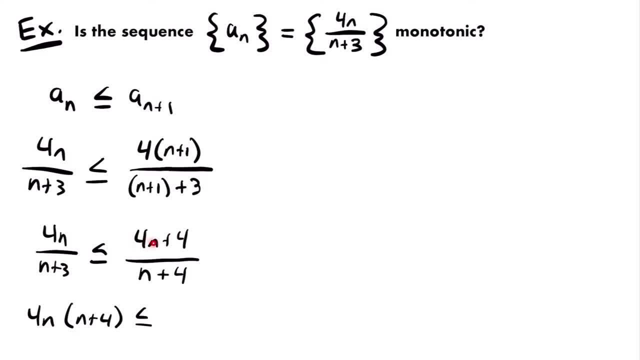 than or equal to n plus 3 times 4n plus 4.. So we have n plus 3 times 4n plus 4.. All right, so all we did was cross multiply, and this was the result of doing that, And so now we can simplify. I'm 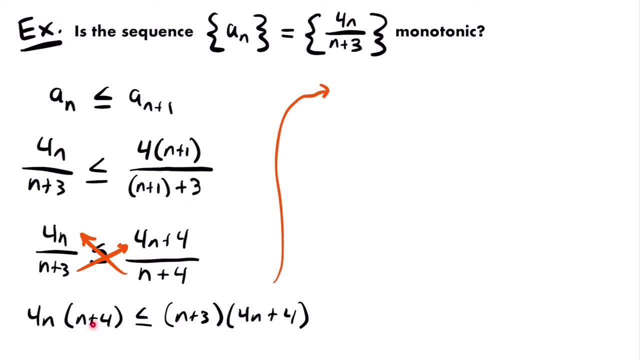 going to continue my work up here. If we distribute 4n through this quantity, we will have 4n squared plus 16n, Right? we multiply 4n by n to get 4n squared, and then 4n times 4n. 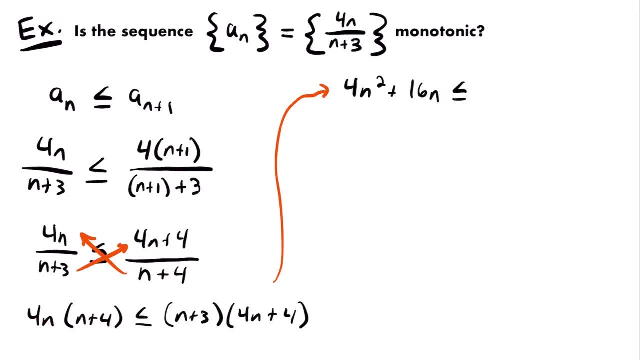 To get 16n, And that's still going to be less than or equal to these two factors multiplied together. Now we need to foil these terms. So what we're going to do is multiply n by 4n, and that will give us 4n squared. Then we'll multiply n by 4, and that will give us 4n, So we have plus. 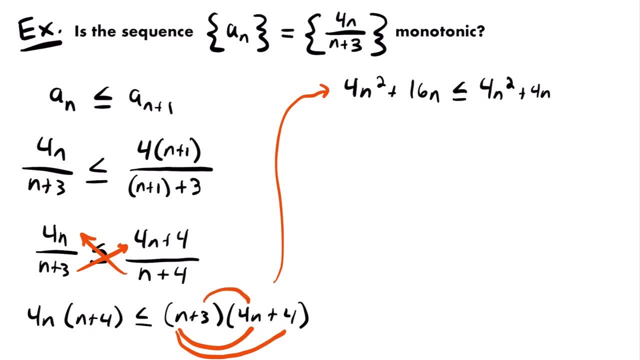 4n, Then we multiply 3 by 4n, So that's equal to 12n, And then we will multiply 3 by 4, and that will have plus 12.. All right, and so now, if we simplify, note that we have 4n squared on both. 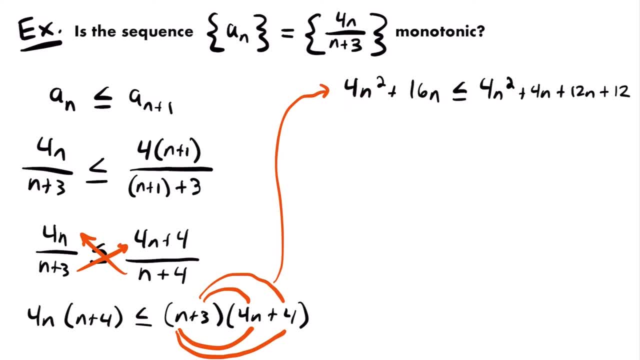 sides of the inequality, And so if we subtract 4n squared from both sides, those are going to cancel out, And so now we just have 16n less than or equal to 4n plus 12n. That's actually equal to 16n. So we have 16n and then plus 12.. All right, now we have 16n on both sides of the. 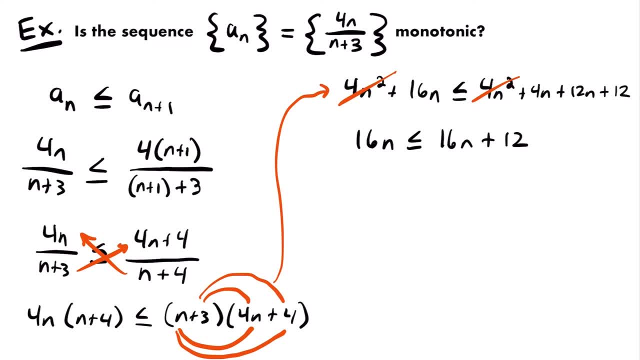 inequality, And so if we subtract 16n from both sides, those will cancel out, And then we'll just be left with 0 is less than or equal to 12.. And so now we have our statement all the way simplified, And now all we have to do is determine if this: 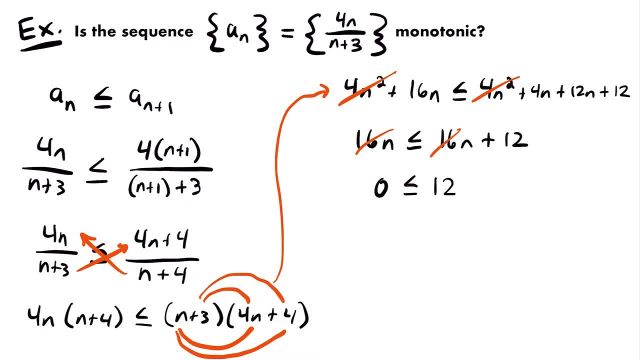 is true. Is 0 less than or equal to 12?? Well, the answer is yes, 0 is less than 12.. And so this is a true statement, which means that we have proved that a sub n is less than or equal to a sub n plus. 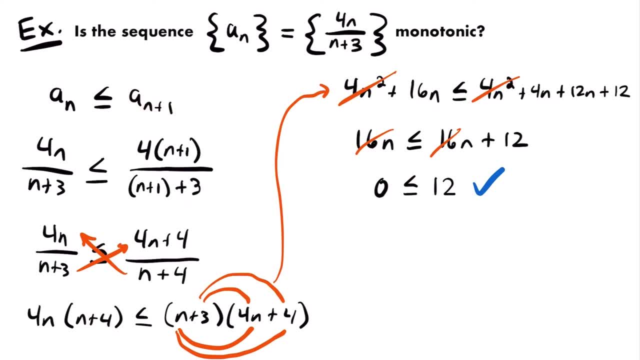 1. Which means that our sequence is increasing, Just as we suspected, And so what we can say is that a sub n is monotonic, And, if you wanted to, you could say that it is specifically increasing. All right, and so that is the solution to this. 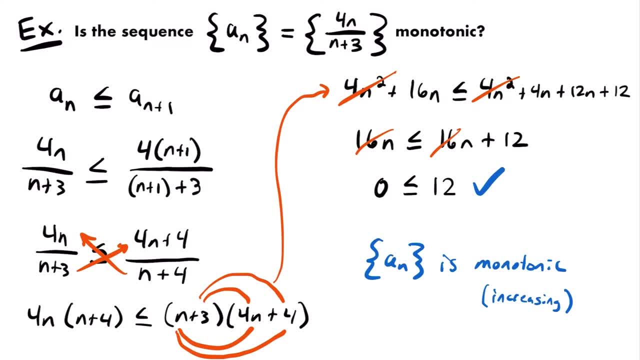 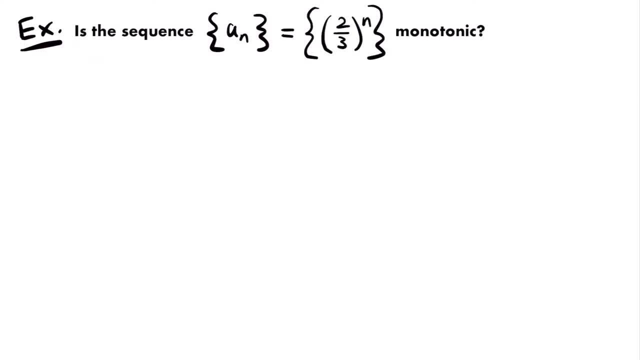 problem. We were able to prove that this sequence is monotonic by showing that its terms are increasing. All right, so here's our next example. We want to know: is the sequence a sub n is equal to two thirds to the power of n monotonic? 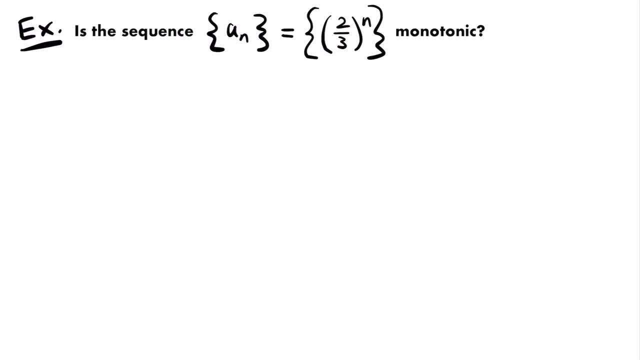 So, once again, we're going to go through that same process. We're going to start by writing out some of the terms of our sequence and see if we can determine if it is increasing or decreasing, And then, depending on what we find, we will then use a general statement to prove that it's either 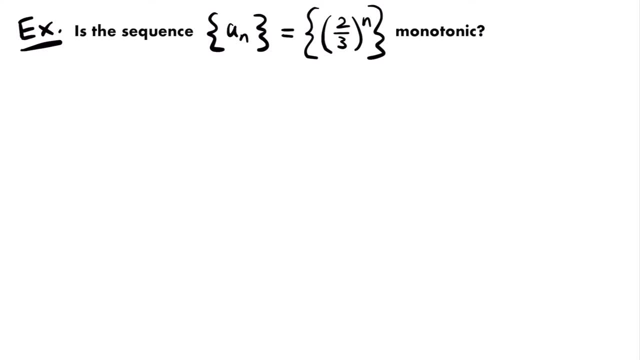 increasing or decreasing. And so let's write out the first couple terms. A sub 1 will be equal to two thirds to the first power. That's just equal to two thirds. A sub 2 will be equal to two thirds squared. So if we square the numerator and the denominator, that's equal to four ninths. Then a sub 3 is going. 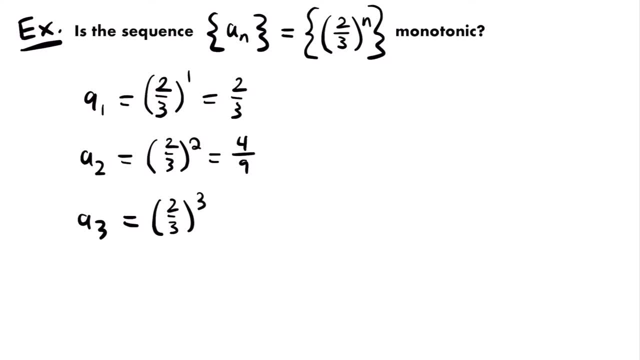 to be equal to two thirds cubed. And if we cube the numerator and the denominator, that's equal to eight twenty sevenths. And then let's look at a sub 4. yet That will be equal to two thirds to the fourth power. And if we take the numerator and the denominator to the fourth power, we will have 16. 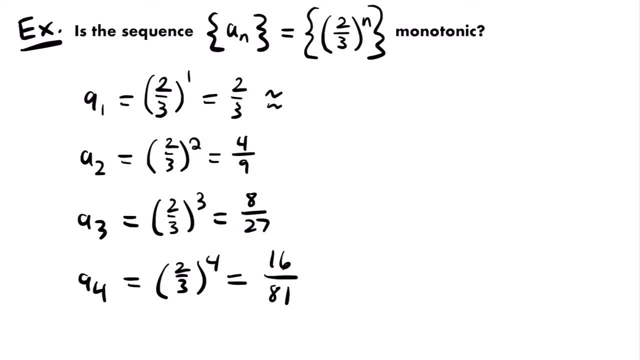 divided by 81. Now, two thirds is approximately equal to zero point six repeating Four ninths is approximately equal to zero point four repeating Eight. twenty sevenths is approximately equal to zero point two, nine, six and some more decimals, And 16 divided by 81 is approximately. 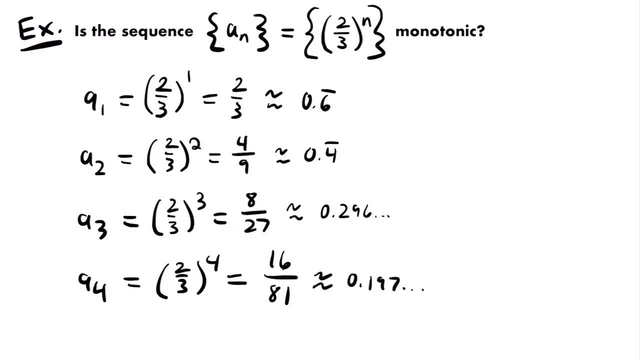 equal to zero point one, nine, seven and some more decimals. And so now, looking at these decimal values, can you determine if our sequence has increasing or decreasing terms? Well, in this case, we started with zero point six, repeating, Then we have zero point four, repeating, Then we 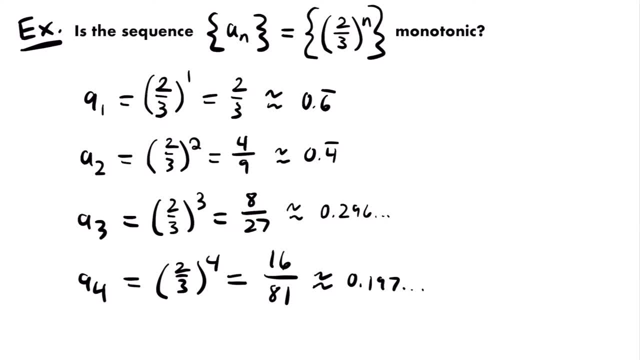 0.296, and then 0.197,, and so each of those terms is getting smaller. Each subsequent term is less than the previous term, And so we can see that our sequence is decreasing. but now we need to prove it, And so we know that if a 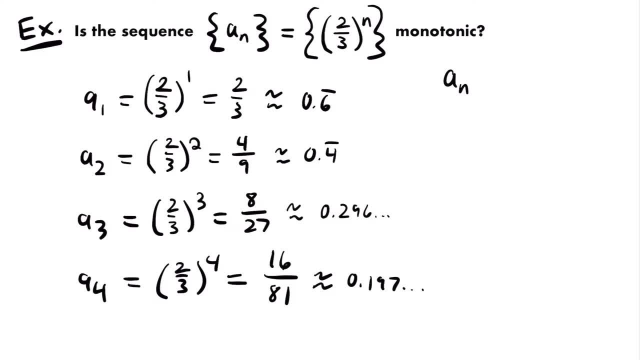 sequence is decreasing that the term- a sub n- is going to be greater than or equal to the next term: a sub n plus 1.. Right, a term is going to be greater than or equal to the next term. We saw that with our terms here. a sub 1 is greater. 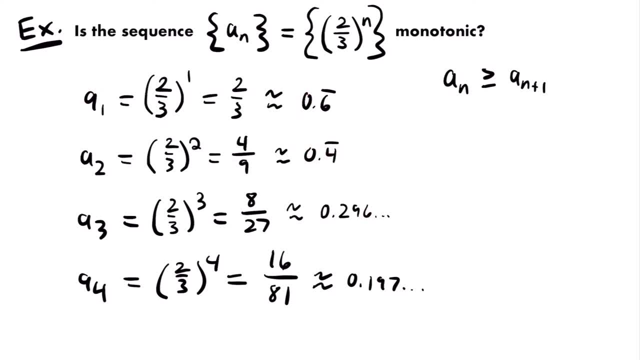 than a sub 2, and a sub 2 is greater than a sub 3.. Each subsequent term gets smaller, and so a sub n will be greater than or equal to that next term, a sub n plus 1.. Now a sub n is 2 thirds to the power of n, and that will be greater. 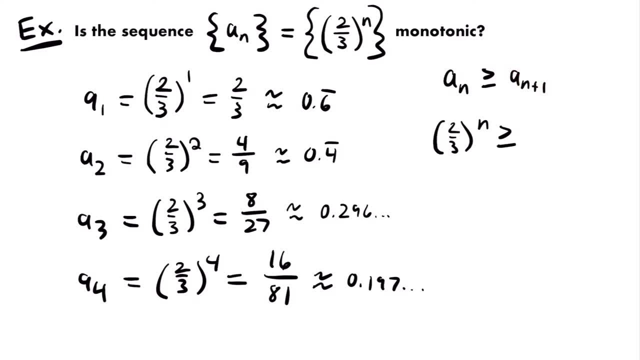 than or equal to a sub n plus 1, so we will replace n in our sequence with n plus 1.. So we'll have 2 thirds to the power of n plus 1.. Okay, so now we want to simplify this inequality and see if we can find a true. 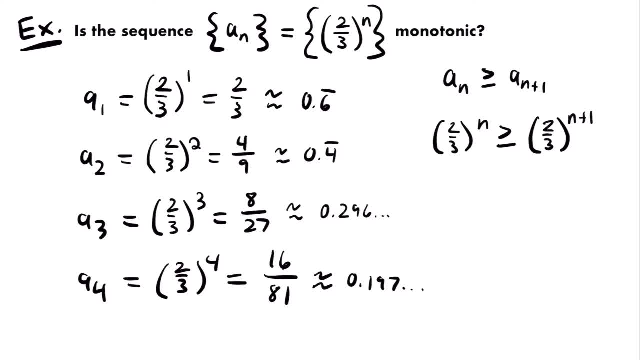 statement. And the way we can simplify this is we can break up this power here. We can rewrite that to be 2 thirds to the power of n times 2 thirds to the power of 1.. Right, when you have the same base raised to an exponent and you 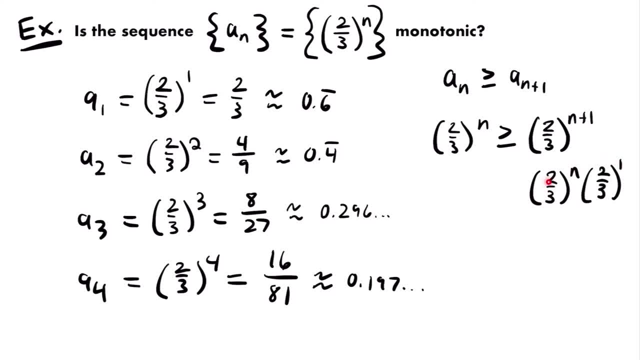 multiply them, you add those exponents. So 2 thirds to the power of n times 2 thirds to the first power would become 2 thirds to the power of n plus 1.. We would add those exponents, And so we can reverse that process by breaking this up. 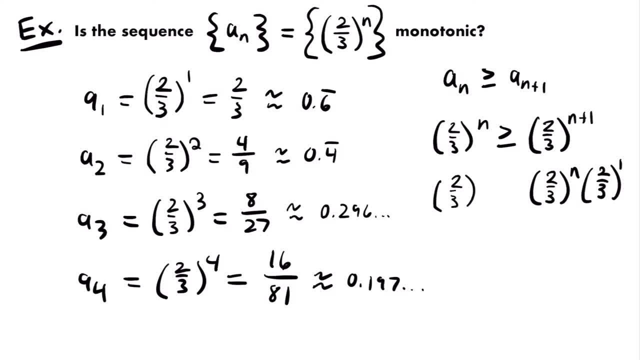 into those two parts, And we're still going to have 2 thirds to the power of n, greater than or equal to that. Now, on both sides of the equation, we have 2 thirds to the power of n, and so what we can do is divide both sides of the. 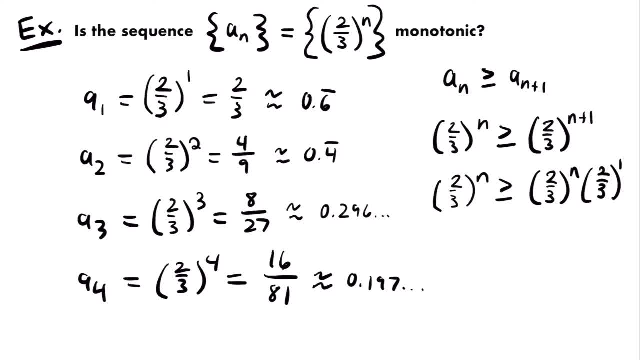 equation by 2 thirds to the power of n, and that will give us that 1 is greater than or equal to 2 thirds. Right 2 thirds is the same as 2 thirds to the first power, and so now we have a. 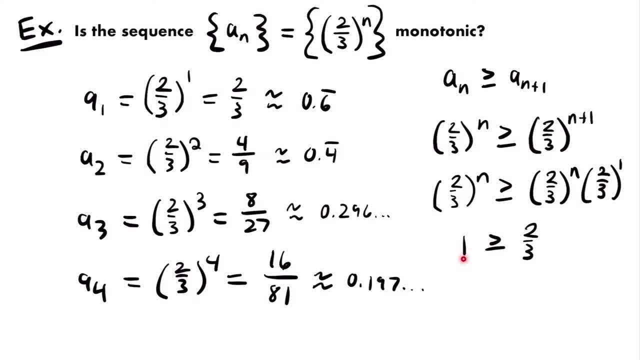 statement that we can check to see if it's true. Is 1 greater than or equal to 2 divided by 3?? And the answer is yes, this is true. 2 thirds is a fraction that is less than 1, and if you weren't quite sure, you could multiply both sides by 3. 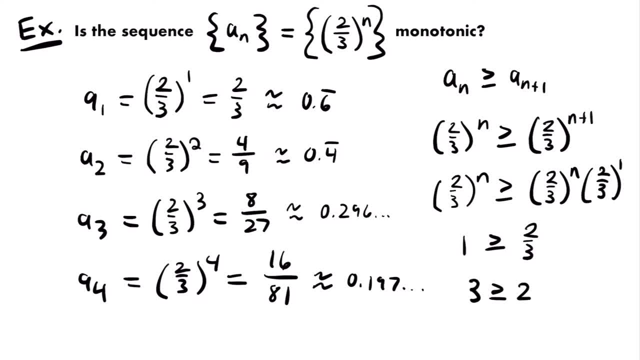 and you would find that 3 is greater than or equal to 2, that is also a true statement: 3 is greater than 2, and so whichever one of these statements you prefer, both are true, and so what we did here is show that this sequence is. 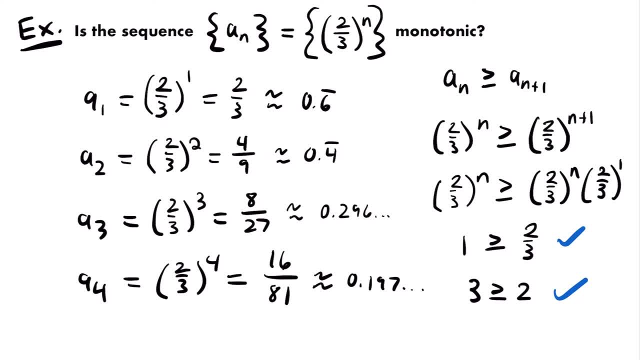 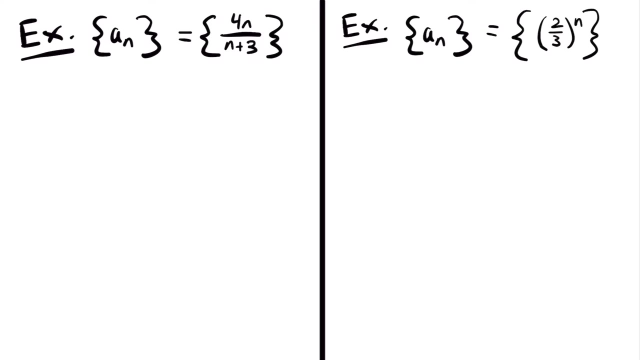 monotonic. Specifically, we showed that it's decreasing, and so, if I erase this last term here, we now know that our sequence, a, sub n, is monotonic. Specifically, it is decreasing. Okay, and so that is the solution to this example. Alright, now, before we end our discussion on monotonic sequences and work our way, 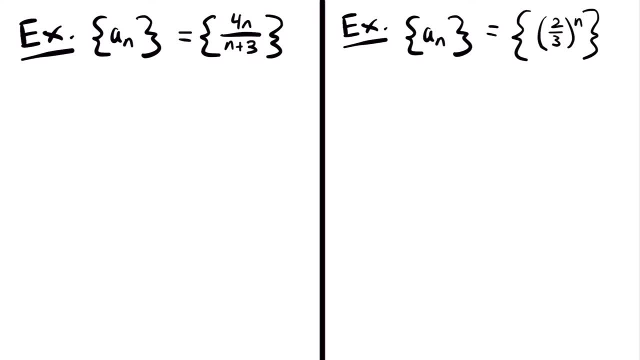 over to bounded sequences. I want to show you an alternative way to determine whether your sequence is monotonic or not. The gangster formula that we use to follow is called the ierra approach, but already kurzweil's basically did that a long time ago, and 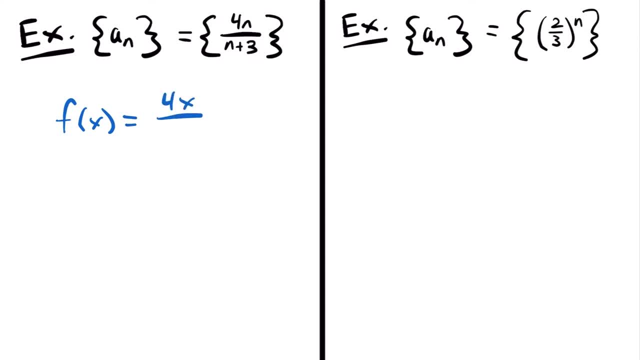 made up theses explanations for when one of the skin groups between the second one and x's is the next one or the second one. In another video we show how, if we So if we took the derivative of this function, f, prime of x, that's going to require the 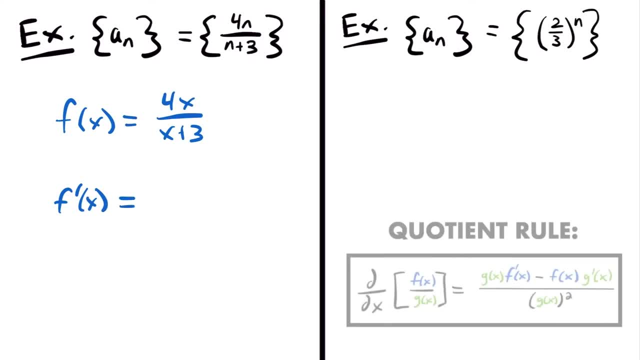 quotient rule, And so if you don't remember the quotient rule, I'll have it up here on the screen for you to reference. But you take the bottom function, which is x plus 3, and multiply it by the derivative of the top function, and so the derivative of 4x is 4, so we multiply by 4.. 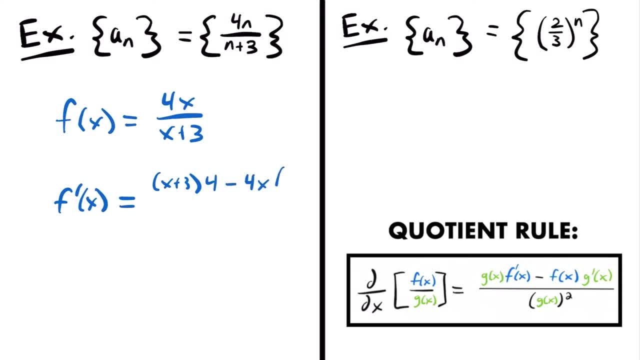 Then we will subtract the top function, 4x, and multiply it by the derivative of the bottom function. So the derivative of x is 1, and the derivative of 3 is 0, so our derivative is just 1.. And then that is divided by the denominator squared. 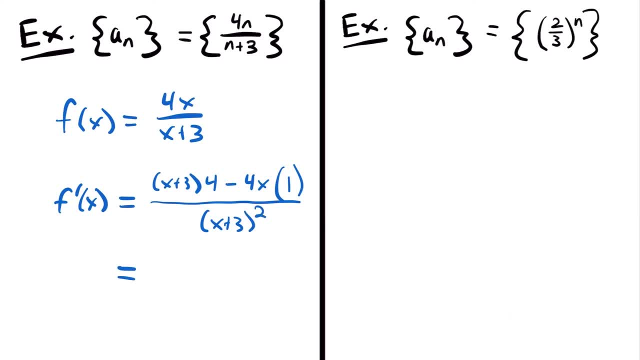 So we have x plus 3 squared, Alright, and so if we simplify, this is equal to 4 times x plus 3, so we have 4x plus 12 if we distribute that 4, and then minus 4x divided by x plus 3 squared. 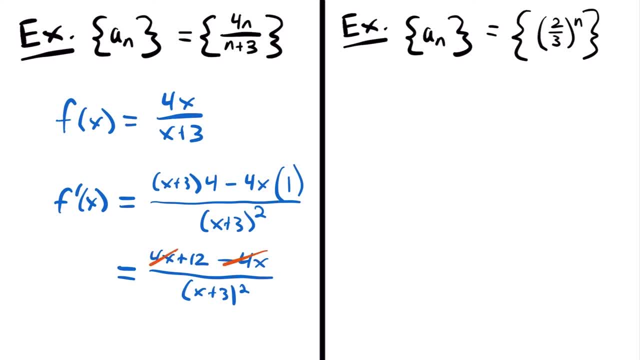 Now we have 4x and negative 4x, so those will cancel out, just leaving us with 12 in the numerator. And so if I erase that, then we can see that our derivative is just 12 divided by x plus 3 squared. 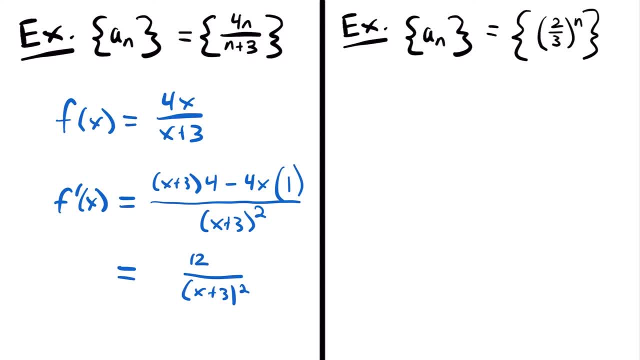 And now the reason we took that derivative is now we can look at the derivative and if it is positive for all values of x, then we can determine that our sequence is increasing. If the first derivative is negative for all values of x, then we can determine that it's 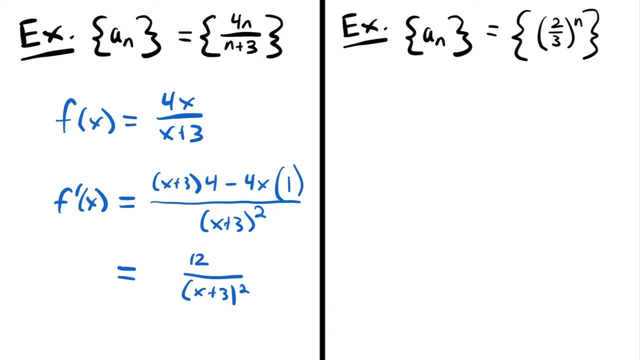 decreasing. Okay, and so in this case we have 12 divided by x plus 3 squared. no matter what value of x you plug in, If we plug into this derivative, this is always going to output a positive value. Right? anything plus 3 squared is going to be positive, because when you square anything, 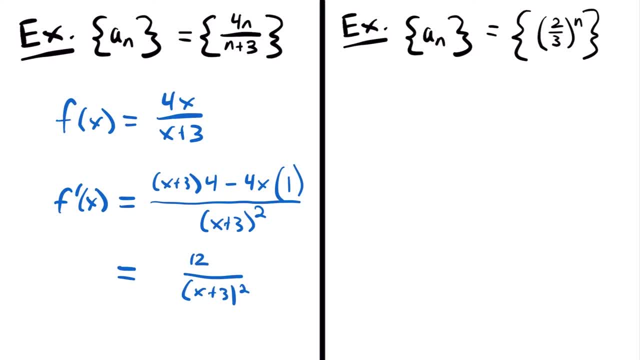 it becomes positive, and then that's just dividing into 12. And so this is always going to be positive, which means that this sequence is increasing, And that's what we found for the sequence earlier in a previous example. we found that this was monotonic because it was increasing. 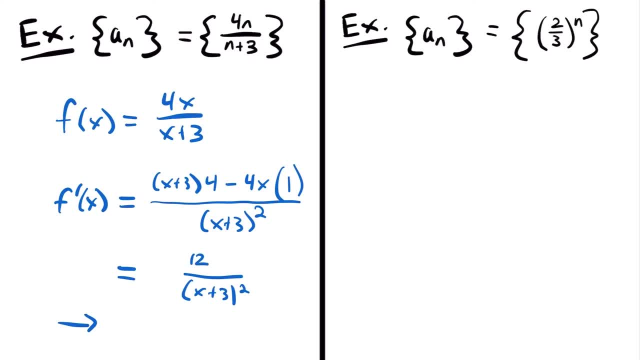 Alright. so since that first derivative is always positive for all values of x and the second derivative is always positive for all values of x, we know that we are increasing, which means that the sequence is monotonic. Now, if we look at our other sequence- this is the other example that we worked on, where 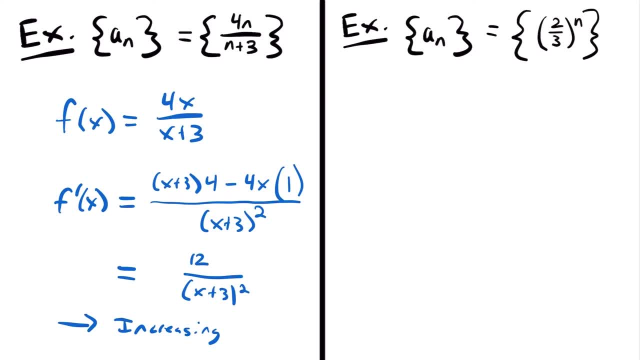 we found it was decreasing. If we take the derivative of the corresponding function to this sequence, we will find that same result: that it's decreasing. Now the corresponding function here would be: f of x is equal to 2 divided by 3, or two. 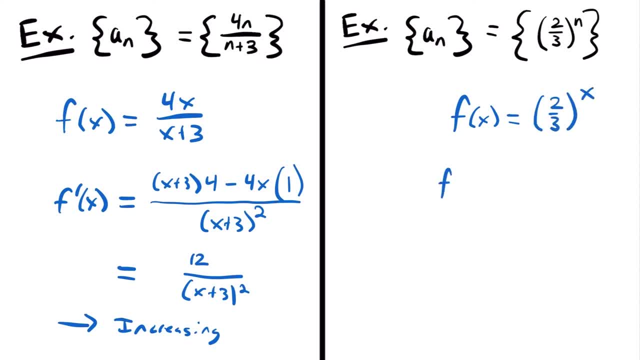 thirds to the power of x And the derivative of that f prime of x will be equal to that exponent. The derivative of an exponential function, two thirds to the power of x times the natural log of two thirds Right, the derivative of an exponential function with a base other than e is equal to that. 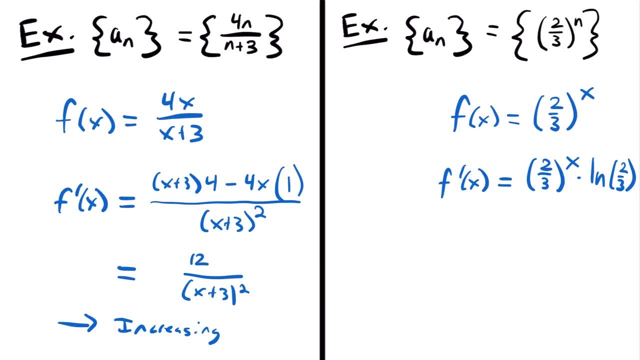 exponential function times the natural log of the base, And so we have the natural log of two thirds. Now, initially this looks like it's always going to be positive, right? We have 2 divided by 3 to the power of x. two thirds to any power of x should always. 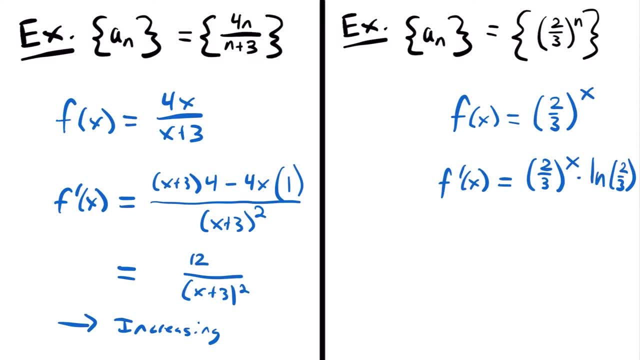 be positive, and then we're multiplying by the natural log of two thirds. However, The natural log of two thirds, if you plug that into your calculator, that's actually equal to approximately negative 0.4054 and some more decimals, And so this constant multiple of the natural log of two thirds is actually a negative value. 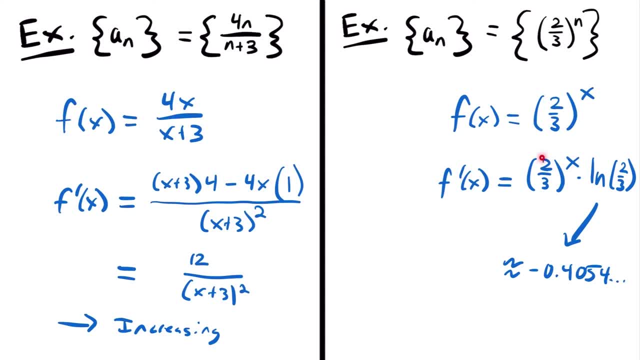 and so that means that we're multiplying that negative value by the result of two thirds to the power of x. And so since this is always going to be positive and we're multiplying it by a value that is always negative, then this whole derivative is going to be negative. 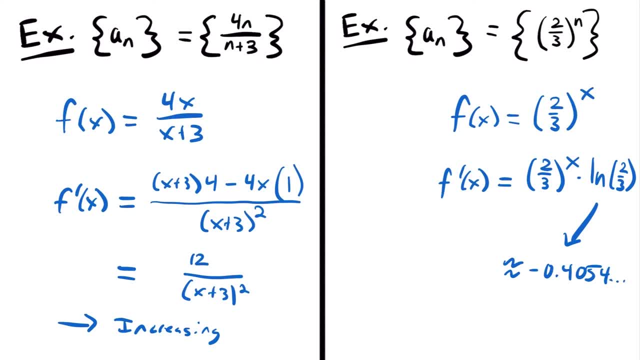 This whole derivative is going to be negative for all values of x, And so what that means is that, since the first derivative is always negative, that our sequence is decreasing. Okay, And so that's another way to come to that same conclusion: that our sequence is decreasing. 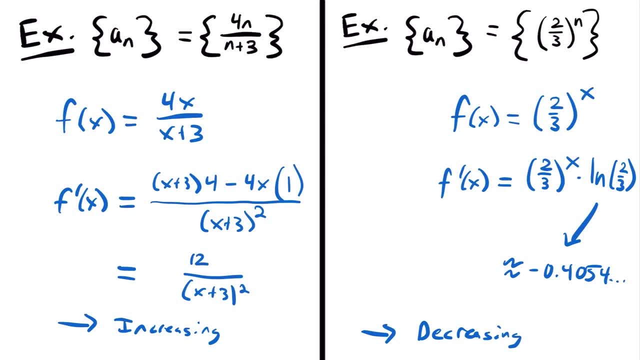 Okay, And so maybe you find this method a little bit easier than the previous method for showing that a sequence is either increasing or decreasing. but typically I prefer the other method where we work with the inequality, But I wanted to show you this method as well. 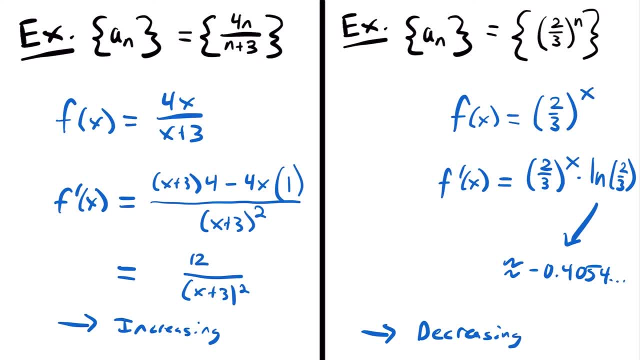 Because it's also valid, and you may prefer this over the other method. Okay, but now, with that, we have established what monotonic sequences are, And so now let's establish what bounded sequences are. Alright, so now we're going to talk about bounded sequences. 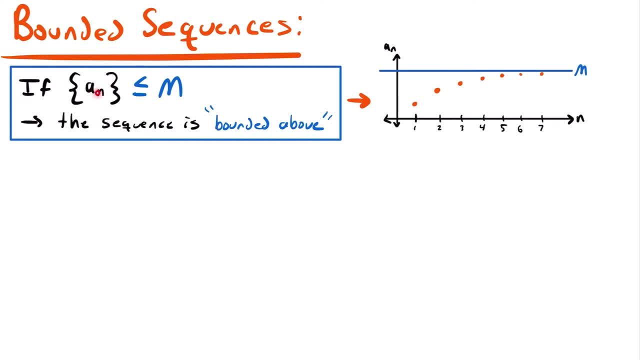 And so the first thing that you need to know is that if a sequence, a sub n, is less than or equal to some value, m, the sequence is bounded above, And so what this means is that all of the terms of the sequence, a sub n, are less than. 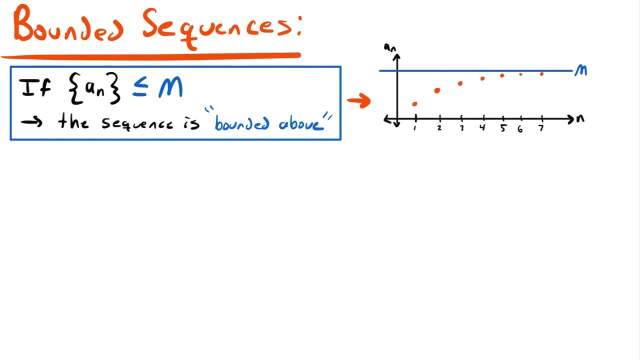 less than or equal to some value, And so visually that looks like this: The terms of our sequence are represented with these red dots and they are bounded above by that value of m, And what that means is that the terms of the sequence will never reach above that value. They are all beneath or equal to that value. 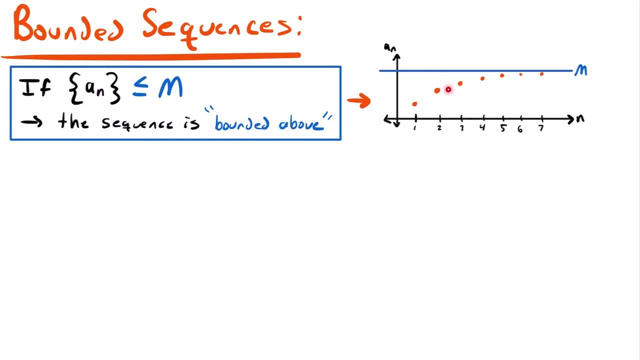 of m, And so if you know that the terms of a sequence are not going to be greater than some value m, then you would say that the sequence is bounded above by that value m. The next thing you need to know is if a sequence a sub n is. 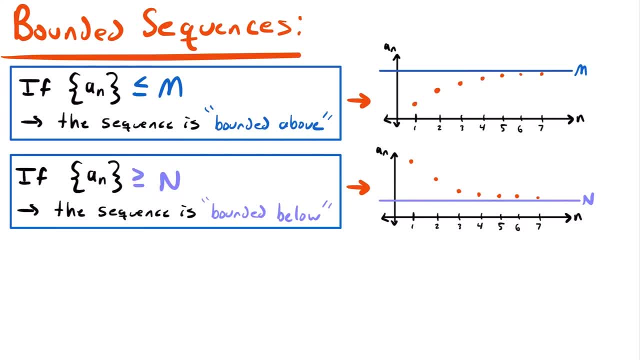 greater than or equal to some value n, then the sequence is bounded below, And so here's what that looks like visually. The red dots, once again, are the terms of our sequence, and they are always greater than or possibly equal to that lower bound of n. They will never get below that value, And so when you see that the 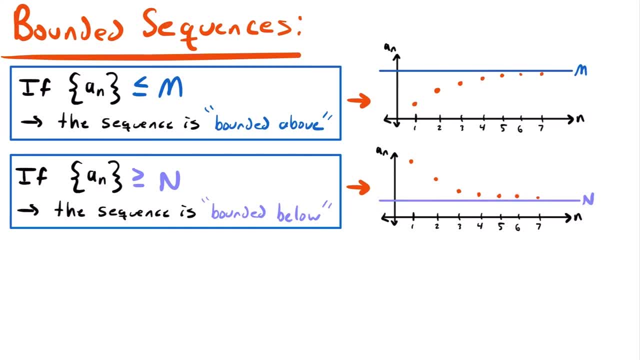 terms of a sequence are always going to be greater than some value or possibly equal to it, then you know that it is bounded below by that value: n. Now finally, if we put everything together, if a sequence is bounded below by n, but bounded above by m, then we say that the sequence is bounded. So, unless the 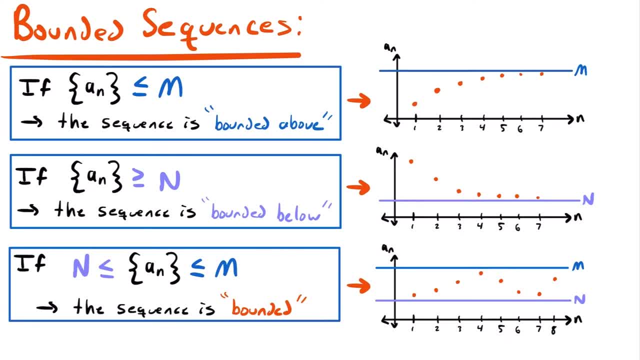 sequence is bounded above and bounded below. it is not bounded entirely. It needs to be bounded both above and below, by some value m and another value n. And so what that means, if you look at this visually, the terms of our sequence, these red dots always. 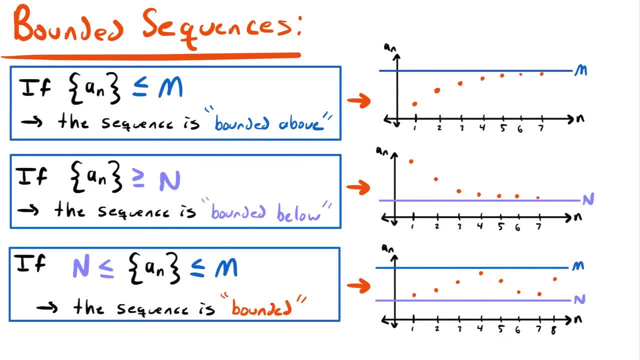 lie between, or are equal to, an upper bound of m and a lower bound of n. They will never go above m and they will never go below n. Now, they could be equal to m or n, but they're never going to be greater than m or less than n. Alright, 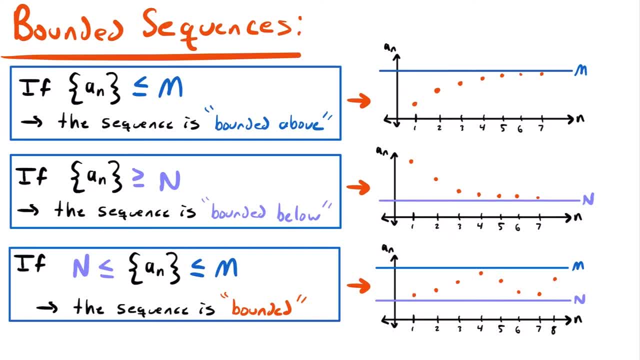 and so if you know that a sequence is going to have terms that will always be less than some value or equal to it, and will also always be greater than or equal to some other value, then you can determine that that sequence is bounded. And so let's take a look at some examples where we determine if a 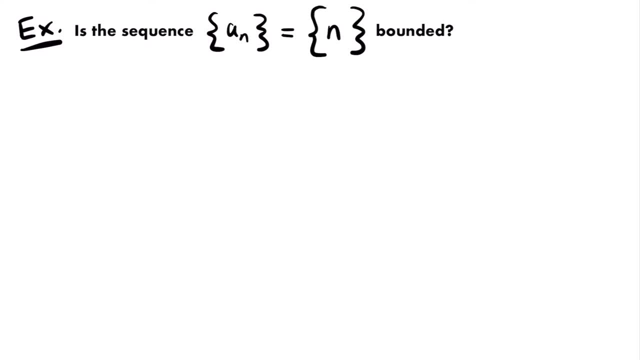 sequence is bounded. Okay, so here's our first example. We want to know: is the sequence A sub n equal to n bounded? And so the first thing you want to do is just determine some of the terms of your sequence. Now, this one's pretty easy: the 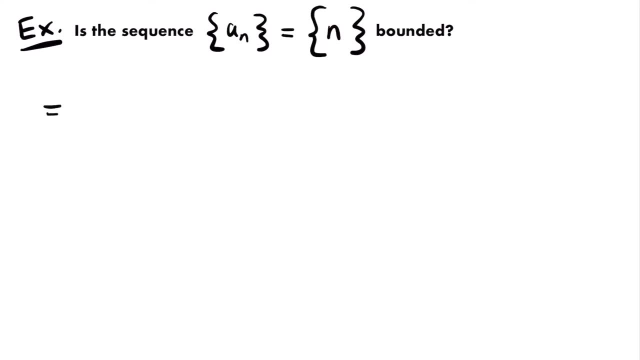 sequence is just n, and so our terms would look like this: A sub 1 is 1, A sub 2 is f is 2, a sub 3 is 3, and then this would continue on forever. right, We're just increasing by 1 each time, and so this is a pretty simple sequence. 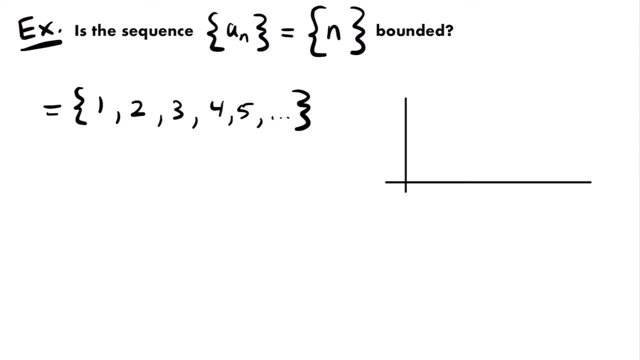 Now, if we were to look at a graph of our terms here, let's draw this out: the horizontal axis will be our values of n and a vertical axis is the value of our terms When n is equal to 1, the value of our term is 1, so that's our first term. 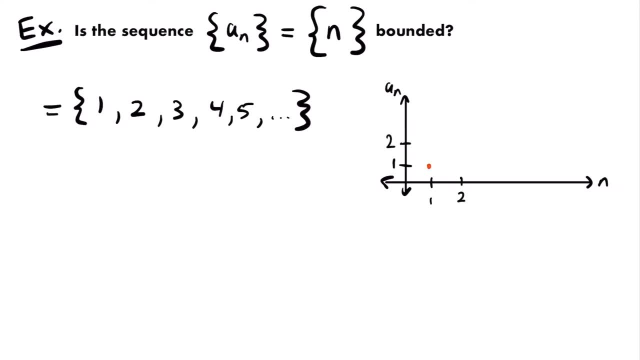 When n equals 2,, then a sub n is 2, so that's our next term. When n is equal to 3,, then a sub n is equal to 3, and so that would be our next term. and you can start to see a pattern here. 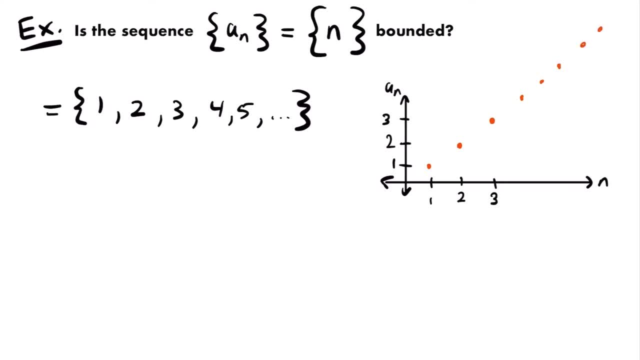 We're just going to continue to increase with these terms forever, no matter what value of n we are at, And so if you look at this graph now, I didn't need to draw all of those points there. but if you look at our terms here, is this sequence going to be bounded above by some value? 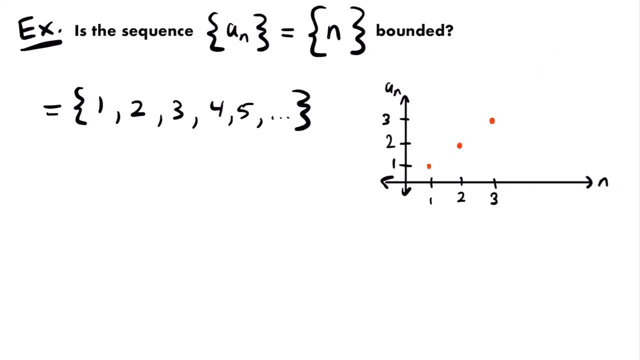 Well, the answer is no. Our terms are going to continue to get greater and greater forever, right? Our terms are 1,, 2,, 3,, 4,, 5, and then it would continue on forever 6,, 7,, 8,, 9,, 10,, 11,, 12,. 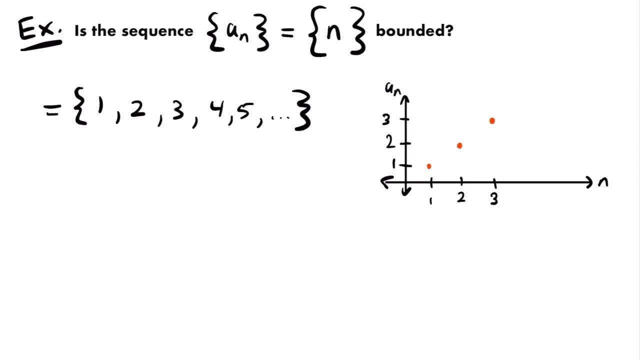 and so on. It's never going to stop at some value. it's just going to keep increasing by a value of 1, and so there's no upper bound m that the terms of our sequence will never go over. They're going to reach every possible value. 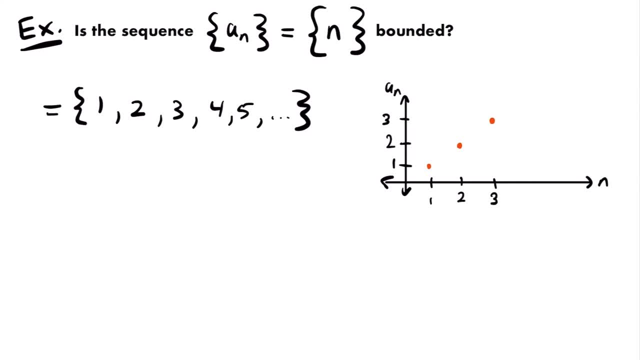 And so the sequence is not bounded above, but it is bounded below, right. When n equals 1,, the term is equal to 1, and we will never have a term less than that value of 1, right, Each subsequent term is just increasing, and so that value of 1 is our lower bound n and 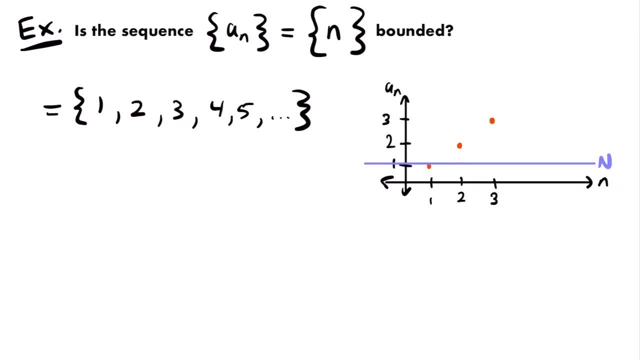 so we would say that this sequence is bounded below by n equals 1.. Alright, so a sub n is bounded below, so that means it's greater than or equal to the lower bound n, which is 1.. And so that means it's bounded below. 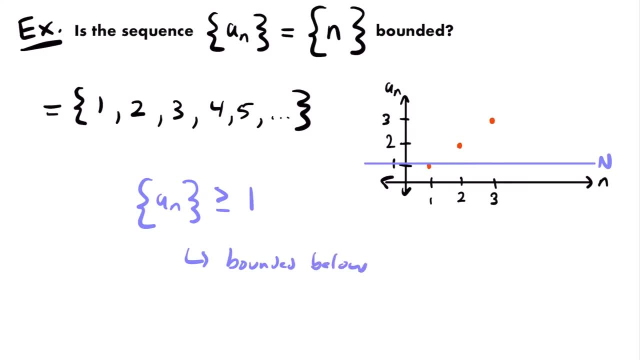 However, it is not bounded completely, because it doesn't have an upper bound. It is not bounded above, And so we cannot say that this sequence is bounded. It's bounded below, but it's not bounded above as well, And so we can conclude that a sub n is not bounded. 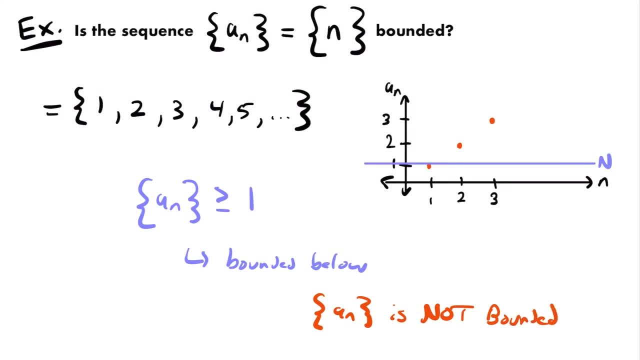 Alright, and if you want to make a note of it, you can say that it's bounded below but not bounded above. Alright, so it might be a good idea to add that to your answer as well. Alright, but our final conclusion is that this sequence is not bounded because it doesn't. 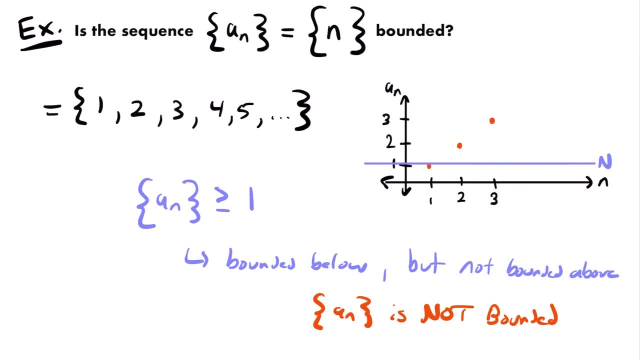 have both a lower bound and an upper bound. It only has a lower bound. Let's look at another example. Alright, here's our next example. We want to know is the sequence: a sub n is equal to 1 divided by n bounded. 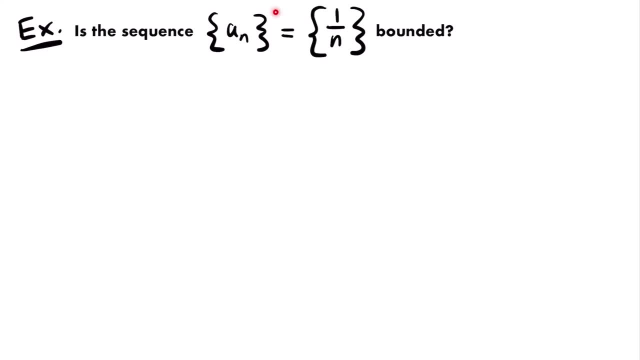 And so let's go through that same process. Let's write out some of the terms of our sequence. first, In this case, we'll have a sub. 1 is equal to 1 divided by 1.. That's equal to 1.. 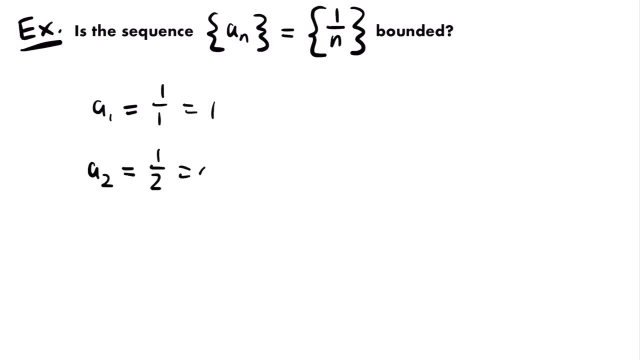 A sub 2 is equal to 1 half, That's equal to 0.5.. A sub 3 will be equal to 1 third, That's equal to 0.3 repeating. And then let's do one more: A sub 4 will be equal to 1 fourth. 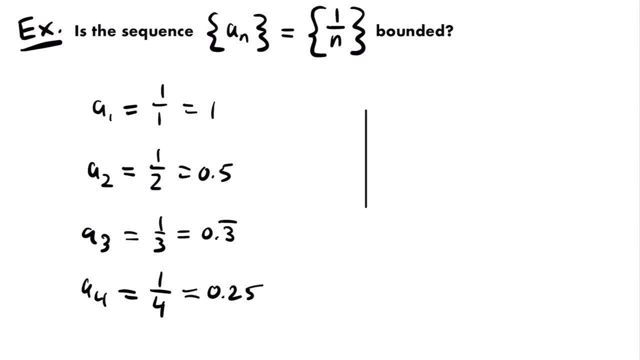 And that's equal to 0.25.. Alright, and so then, if we were to graph out these terms of our sequence, remember that our horizontal axis are the values of n and our vertical axis are the values of our terms. a sub n. 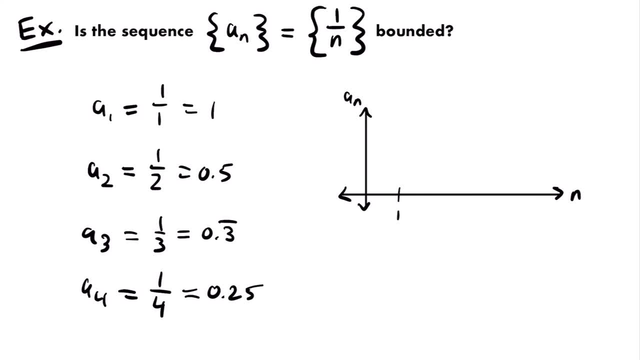 So we're just going to graph our first four terms here, And so we'll have: n is equal to 1, n is equal to 2, n is equal to 3, and n is equal to 4.. Now, when n is equal to 1,, the value is equal to 1.. 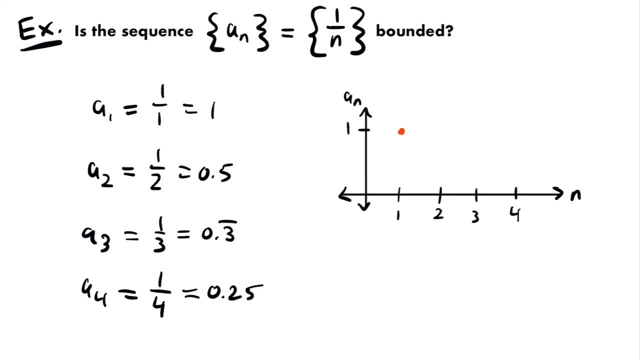 That is the value of our term. So that will be our first term. Then, when n is equal to 2, we have 0.5.. So that will be our next term. Then, when n equals 3, we have 0.3. repeating. 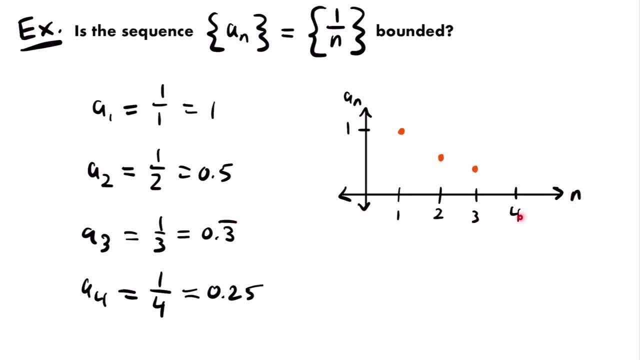 And so that will be right about here somewhere. And then, when n is equal to 4, it's equal to 0.2. Which will be right about here. Alright. now, by looking at the graph of these terms, can we conclude that this sequence: 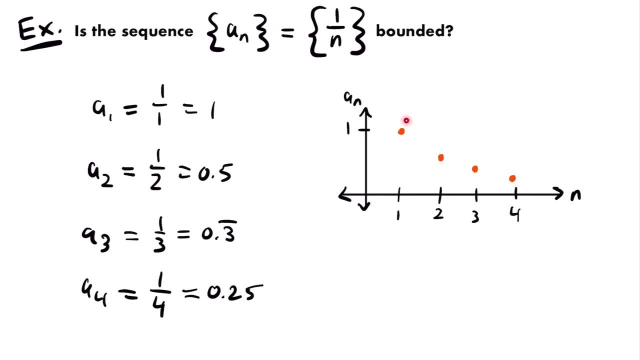 is bounded. Is there some upper bound that these terms will not get greater than? And is there some lower bound that they will never go below or be less than? Well, let's start with the upper bound. We can see from these terms that they are progressively getting smaller towards 0.. 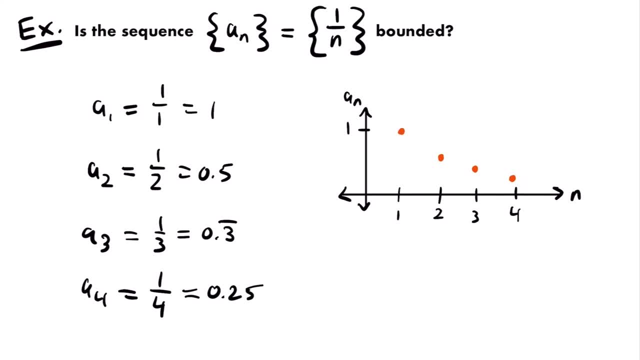 And so they're never going to be greater than the initial value of the first term, And that is that a sub 1 is equal to 1.. So we could say that at that value of 1, the sequence is bounded above, That is the value of m. 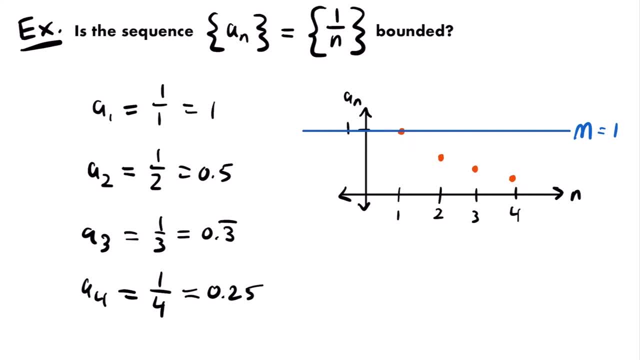 m will be equal to 1.. Our terms are never going to be greater than that value of m, And so our sequence, a sub n is bounded above by m, And that's equal to 1.. So I'm just going to erase m and write 1.. 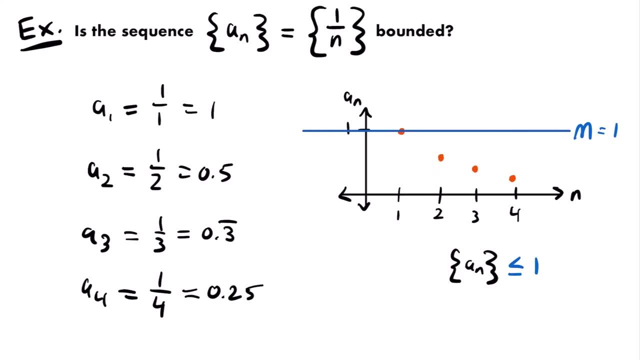 But now let's see if it's bounded below And if you look at the terms on our graph, You can see that they're appropriate. They're approaching 0.. But if we think about this logically, our sequence is 1 divided by n. 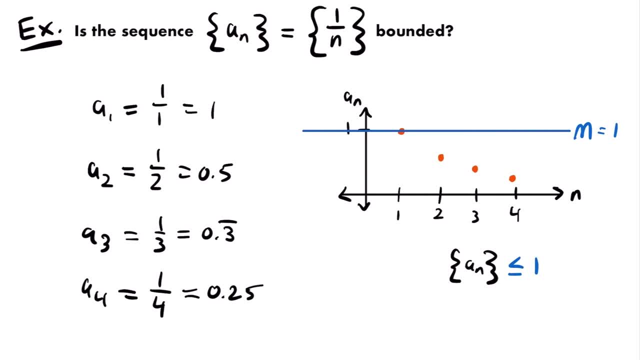 And n is only going to be positive integers, starting at positive 1.. And so this sequence is always going to output a positive value: 1 divided by n will never be negative, since n starts at positive 1.. And so all of our terms we know for a fact are going to be positive. 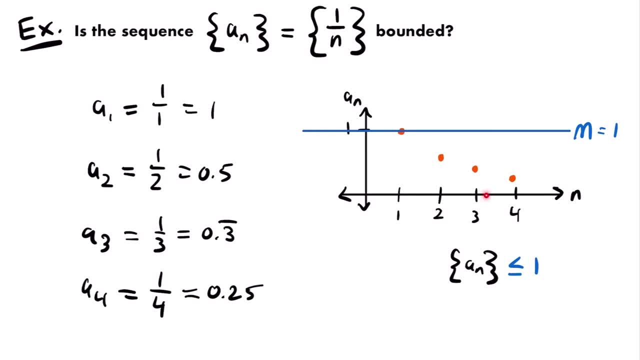 They're going to be greater than 0. And so they will never reach below 0. And so we can say that our lower bound will be 0. And so n is equal to 0. Our terms are never going to go below that lower bound. 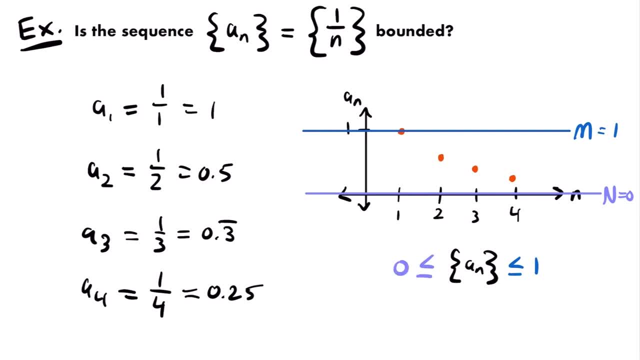 And so we can say that our sequence is bounded below by 0.. Alright, so our sequence, a sub n or 1 divided by n, is bounded above by 1 and bounded below by 0.. And since it has both an upper bound and a lower bound, the sequence itself is bounded. 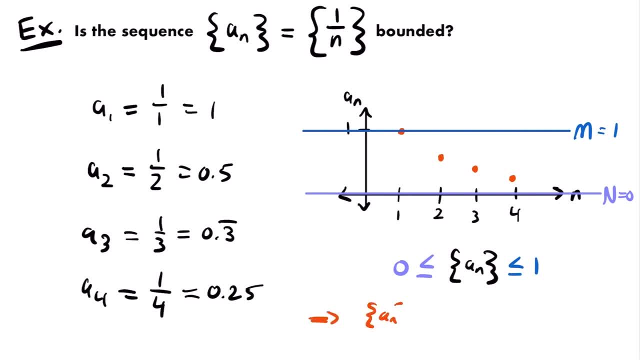 Okay, And so we can conclude: Okay, So a sub n is bounded. Alright, that is the final solution to this example. Alright, and so that's the last example where we focus just on if a sequence is bounded or not. But now we're going to come full circle and revisit that theorem from the beginning. 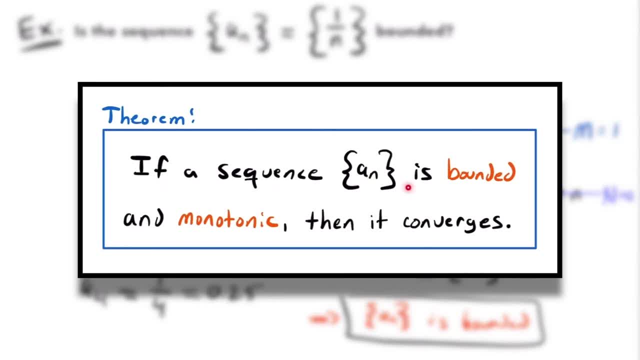 Remember, I showed you this theorem that if a sequence, a sub n, is bounded and monotonic, then it converges. And so now that we know what it means for a sequence to be bounded and to be monotonic, we can test both of those things for a sequence and determine if it converges without ever. 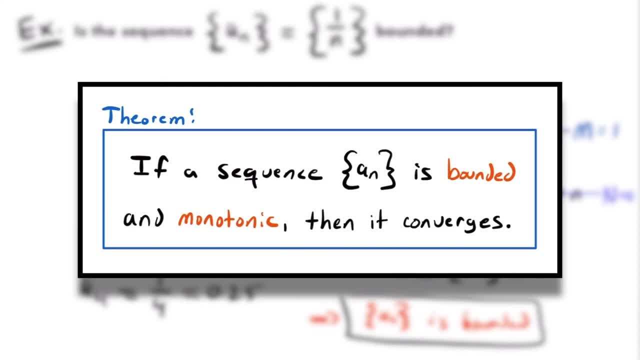 needing to use a limit, And the reason we would want to do this is that it might be an easier method for determining the convergence of a sequence when the limit method may not be the preferred method, where it might be a little bit more difficult than you would like it to be. 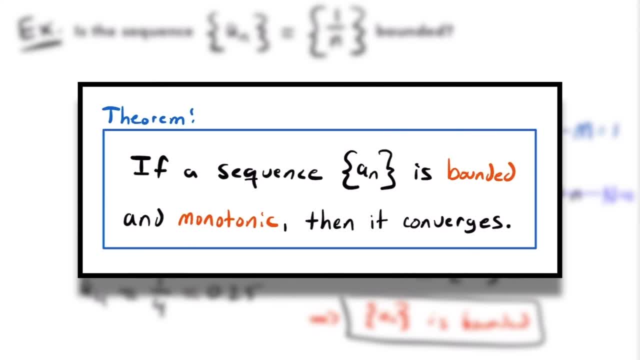 And so this might be a nicer way to show that a sequence converges. And so let's take a look at an example where we have a sequence and see if we can determine if it converges Based on if it's bounded and monotonic. 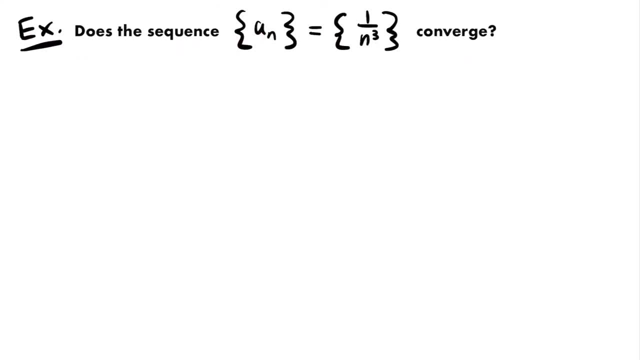 Alright, so here's our first example. Does the sequence a sub n is equal to one divided by n cubed converge? And so the way we want to determine this is see if our sequence is both monotonic and bounded. And so let's start by seeing if our sequence is monotonic, and then we'll work on if it's. 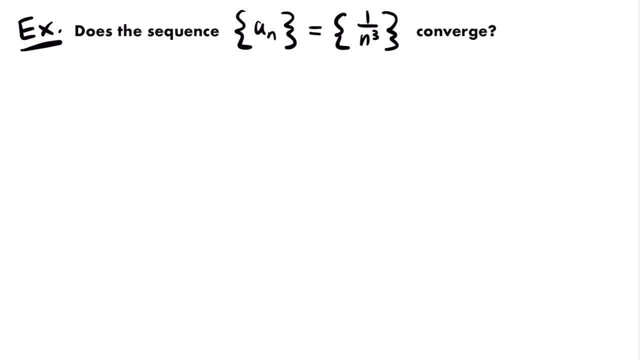 bounded or not, And so we'll start by writing out the first four terms or so of our sequence. So we know that a sub one will be equal to one. Let's say that a sub n is equal to one divided by one cubed, and that will be equal to one. 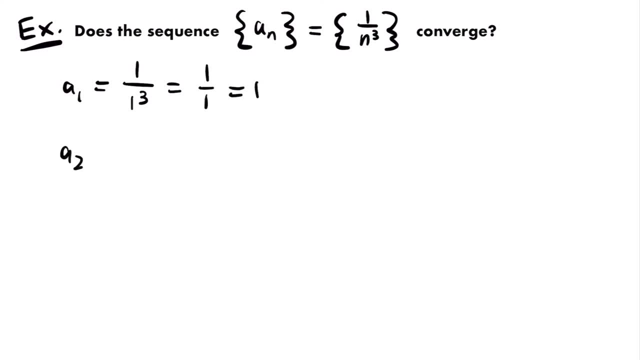 divided by one, which is equal to 1.. A sub 2 will be equal to one divided by two cubed, and that will be equal to one eighth, and that is equal to 0.125.. A sub 3 will be equal to one divided by three cubed, and that's equal to one twenty-seventh. 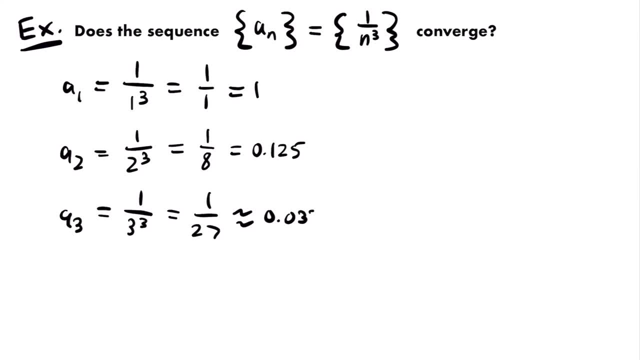 and that's approximately equal to 0.037, and some more decimals. And then let's do one more: a sub 4 will be equal to 1 divided by 4 cubed, which is equal to 1- 64th, and that is equal. 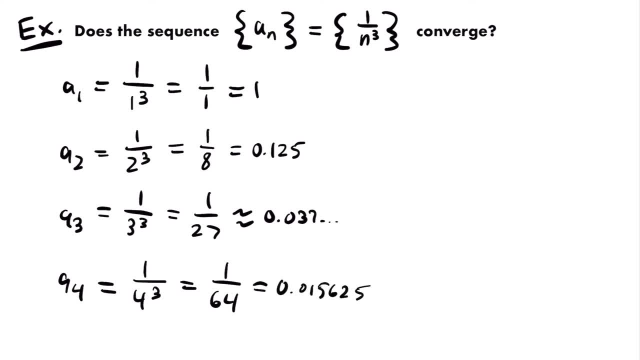 to 0.015625.. Alright, now, by looking at these terms, can we see if it's increasing or decreasing? Remember, that's what we're looking for. if we want to determine if our sequence is monotonic, We want to look to see if our terms are increasing or decreasing, and in this case it looks like. 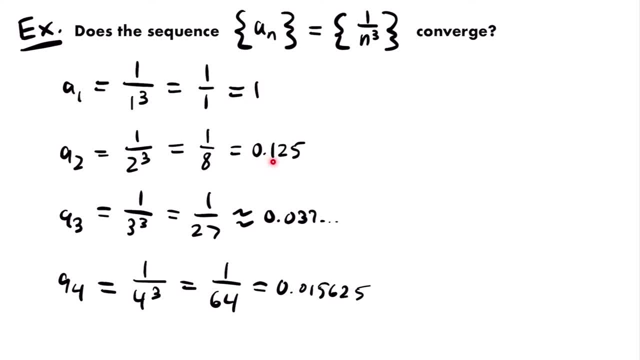 they are decreasing. We started with 1, then we have 0.125, which is less than 1, then we have 0.037, which is less than 0.125, and then our next term is even smaller: 0.015625 is less than 0.037.. 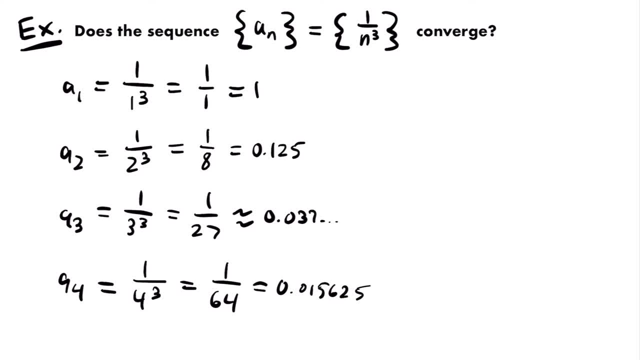 And so each subsequent term is decreasing, and so let's try to prove that this sequence is decreasing by using one of our statements. So, since we want to prove that it's decreasing, that means that a term, a sub n, will be greater than or equal to the next term. 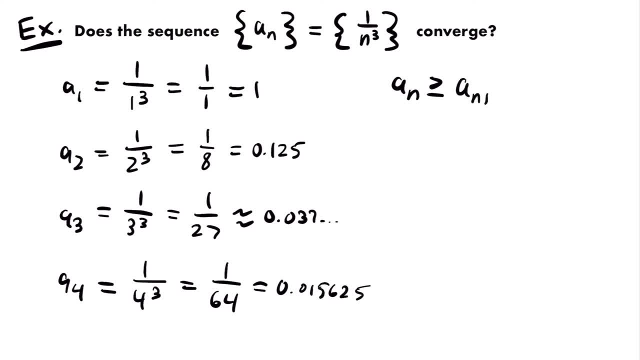 The next term, that's going to be smaller, which will be a sub n plus 1.. And so let's look at a sub n and a sub n plus 1. for our sequence, A sub n is just 1 divided by n cubed, and that will be greater than or equal to 1 divided. 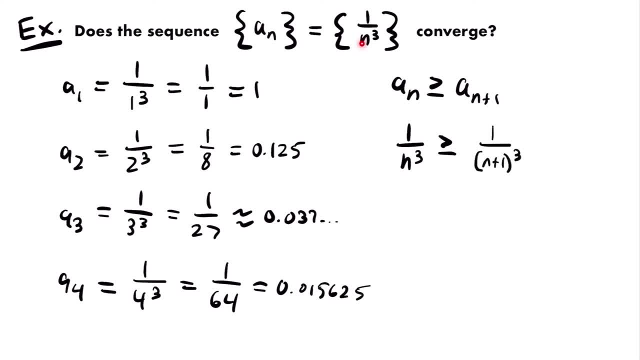 by n plus 1 cubed. We just replaced n with n plus 1, so we have 1 divided by n plus 1 cubed. Now if we simplify this expression, let's cross multiply, so we'll multiply n plus 1 cubed. 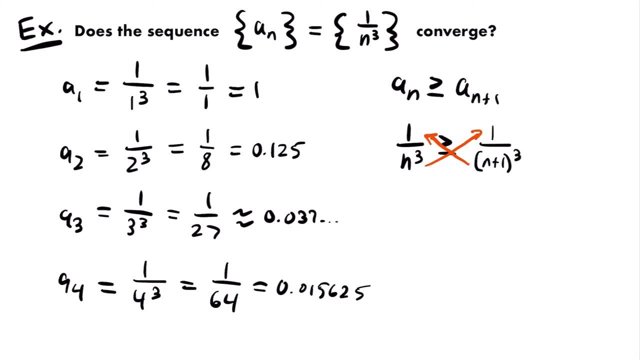 by 1 and n cubed by 1.. And that will give us n plus 1 cubed greater than or equal to n cubed. And now, if we take the cubed root of both sides of this inequality, we will have n plus. 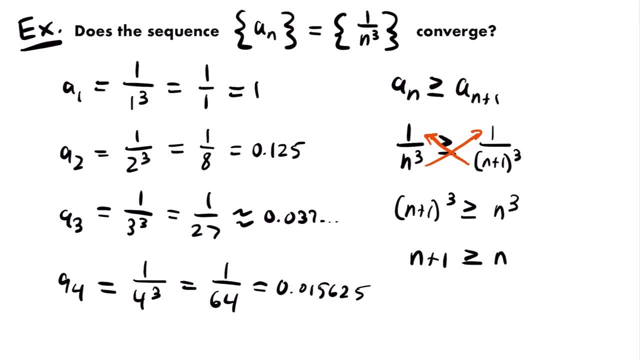 1 is greater than or equal to n, And now hopefully you can see that n plus 1 is always going to be greater than or equal to n. If you're adding 1 to n, it's obviously going to be greater than n, but if you're not sure, 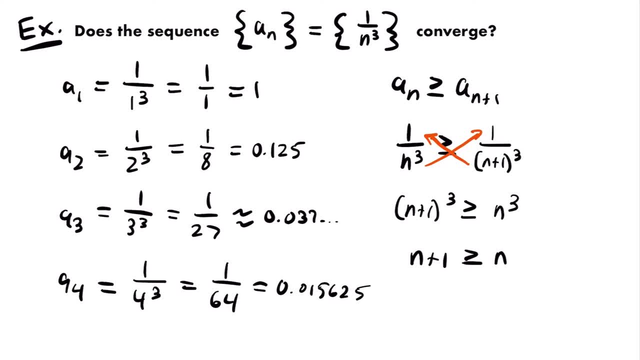 you can subtract n from both sides of the inequality and you'll have: 1 is greater than or equal to 0. And that is also true, And so, since both of these statements are true, we can conclude that this sequence is decreasing, meaning that it is monotonic. 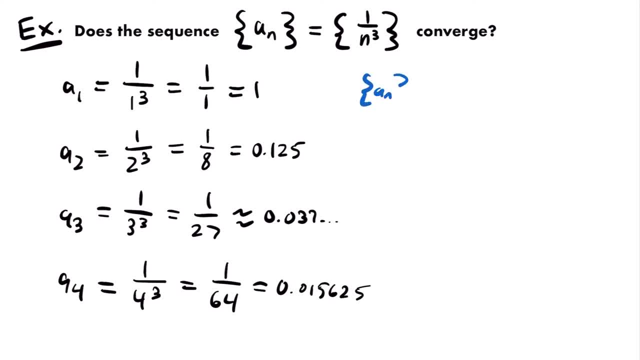 And so, if I clean up my work here, we proved that a sub n is monotonic. Specifically, we showed that it was decreasing. Alright, so that's one half of the problem. In order to determine if this sequence converges, it first needs to be monotonic. 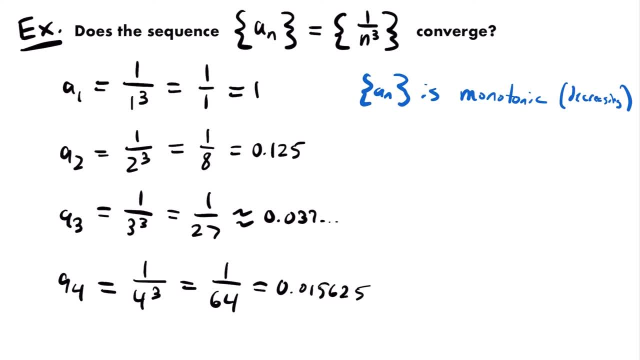 And we found that that was true. So that's good, But it doesn't converge until we also prove, or also show, that it is bounded. And so let's graph these terms here, Let's look and see what happens to our terms visually. 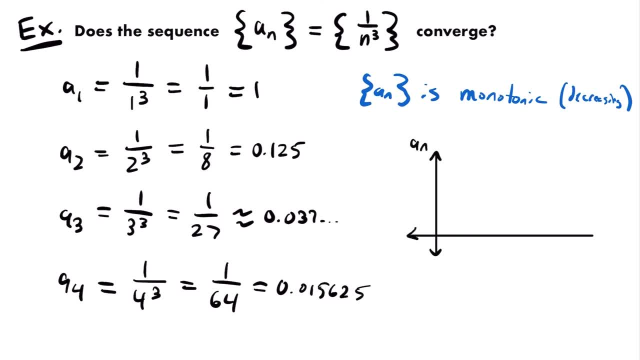 Remember that our vertical axis is the value of our terms and the horizontal axis are the values of n, And so we have 4 to work with here. n equals 1,, 2,, 3, and 4.. And when n is equal to 1, a sub 1 is equal to 1.. 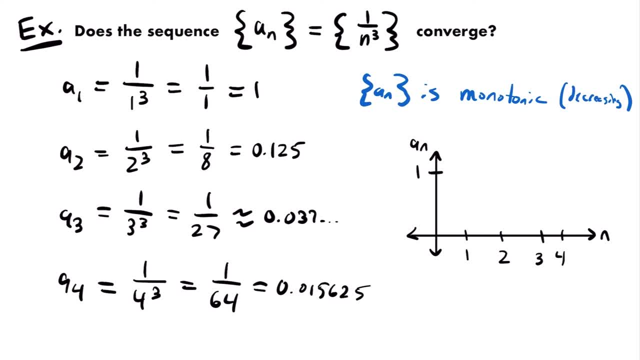 And so this will be our value of 1.. And so this will be our value of 1.. And so this will be our value of 1 for our terms. So this is a sub 1.. Then a sub 2, or when n is equal to 2, that's equal to 0.125.. 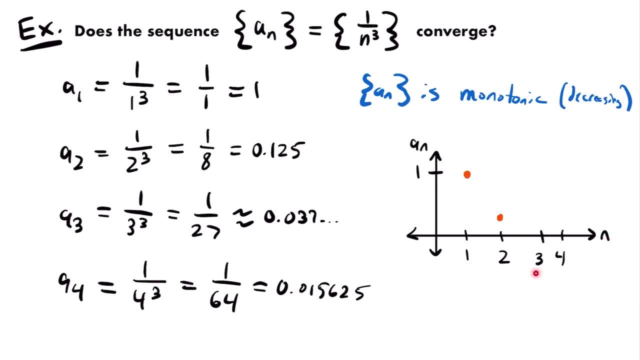 So that's going to be way down here somewhere. And then when n equals 3, it's even smaller than that. So that will look like this: And then n equals 4 or a sub 4 is going to be even smaller, And so you can see from this graph that our sequence is decreasing, like we determined. 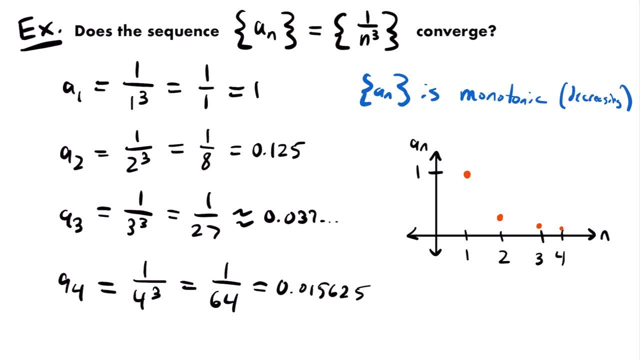 But is there an upper and lower bound for this sequence? Well, similar to one of our previous examples for looking at bounded sequences, 1 divided by n- cubed, this sequence is always going to be positive, right? We're only plugging in values of n, starting at positive 1 and then increasing towards. 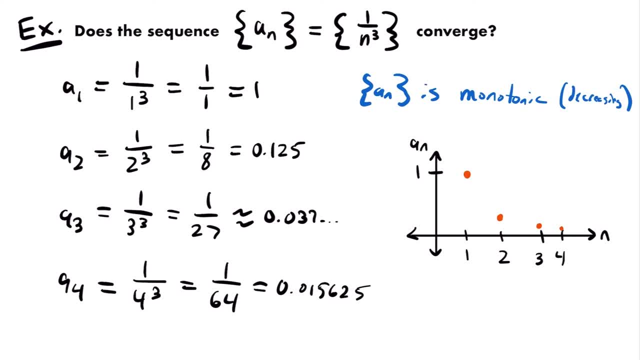 infinity, And so we're never going to be plugging in any negative values to this sequence. So this sequence is always going to produce a positive term, which means that our terms are always going to be greater than or equal to 0. They're never going to be positive. 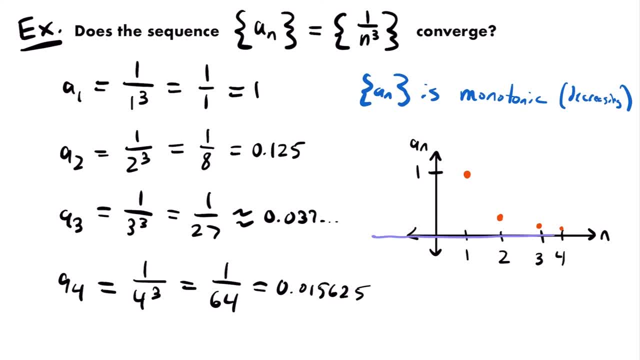 They're never going to drop below 0.. And so we have a lower bound of n, specifically at 0.. So our lower bound is: n is equal to 0.. So we would say that our sequence, a sub n, is bounded below by 0.. 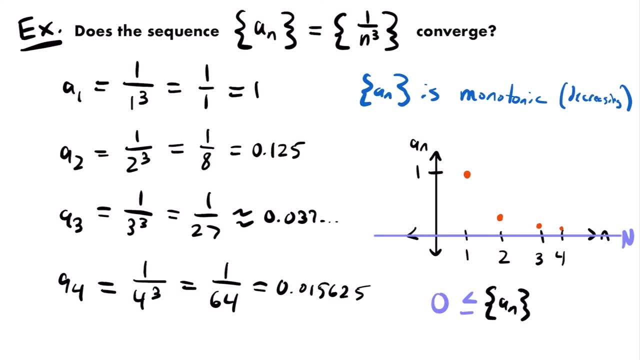 It is always greater than or equal to that value. But then what about an upper bound? Does our sequence have an upper bound? And the answer is yes. Our first term: a sub 1, which is equal to 1, right, that is the highest value of a term. 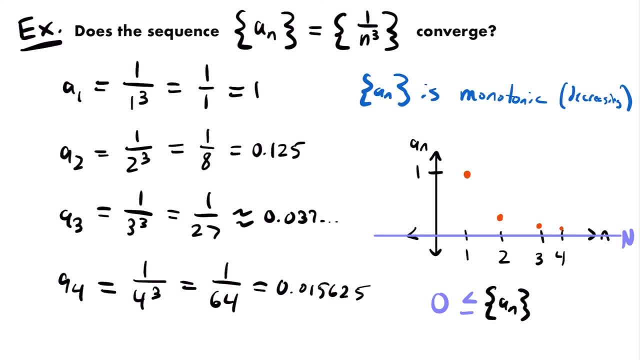 that we will ever have. We already proved that our sequence is decreasing, And so it's never going to come back up above 1.. It's going to continue to decrease for all values of n, And so 1 is the highest value that a term will ever be. 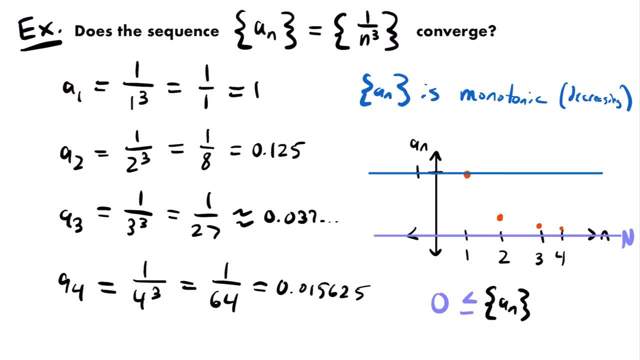 And so we can say that 1 is the upper bound of our sequence, That is, m. The terms of our sequence will never be greater than m, And so they are less than or equal to that value of m which is 1.. 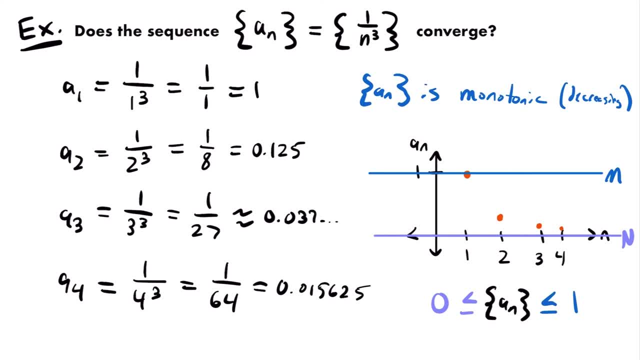 So our sequence is less than or equal to 1.. And so we have a lower bound. And so what we find here is that our sequence is bounded below by 0 and bounded above by 1.. And since it is bounded below and above, we can say that it is bounded. 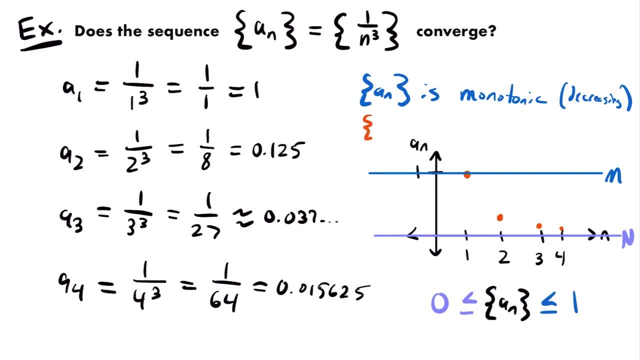 And so not only is a sub n monotonic, but a sub n is bounded. And so, since we determined that it's monotonic and it's bounded, that means that this sequence does converge. Now, we weren't asked to find the specific value that it converges. 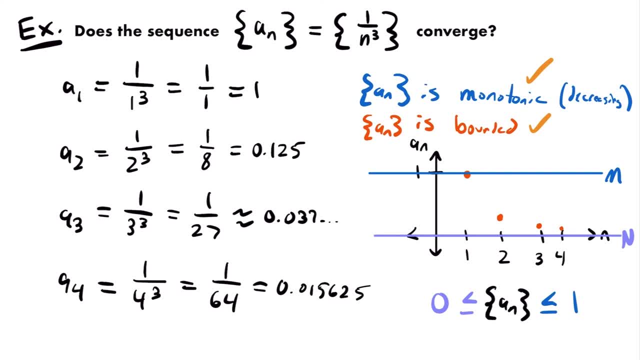 We didn't. We weren't asked to find the specific value that it converges to. We were just asked: does it converge at all? And so we've answered that question, And so I'll just write down our answer: A sub n converges. 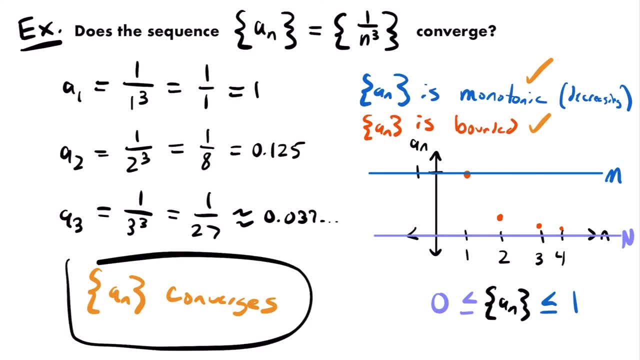 And so that is the final answer to this problem. Now, if you were asked to find the specific value that it converges to, then maybe you would need to bring out a limit to show that it does converge to 0.. And you can kind of see that from our graph, that our terms are getting closer and closer. 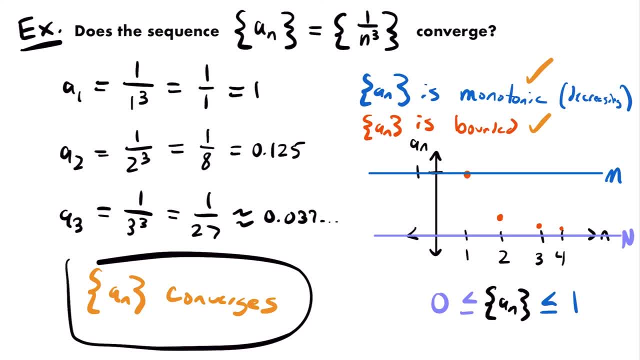 to 0.. So that's what it converges to, But we're not asked to determine. We're not asked to determine what it converges to, just does it converge in general. And so we were able to determine that by showing that a sub n is monotonic and a sub n is bounded. 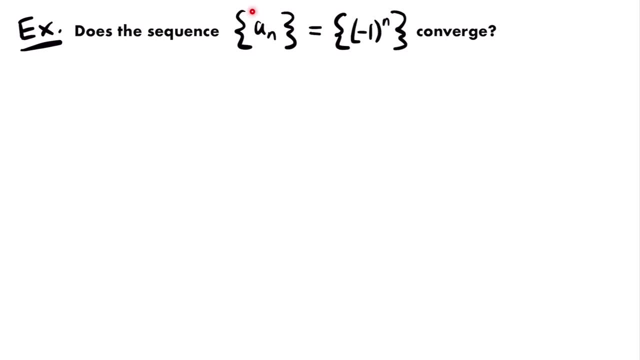 Let's look at one more example for this lesson. All right, so here's our last example. We want to know: does the sequence a sub n is equal to negative, 1 to the power of n converge? All right, and so the first thing we want to do is write out some of the terms of our 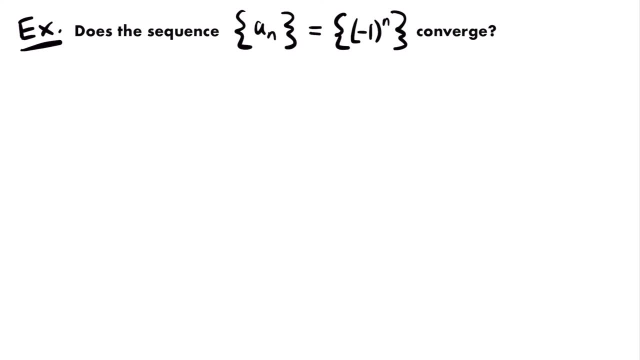 sequence and we'll use those terms to determine if it's monotonic or not. We'll start with that And then we'll talk about whether it's bounded And so negative 1 to the power of n. this is a pretty common sequence that you're probably 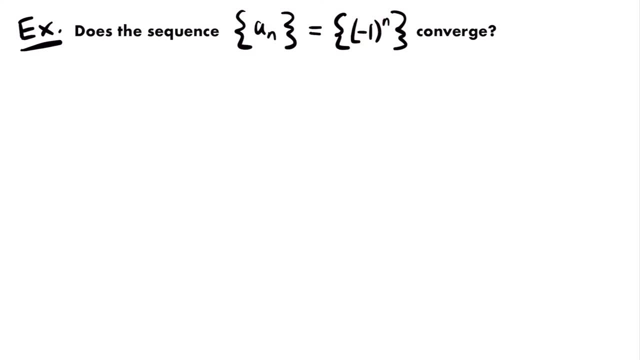 used to. by now We know that negative 1 to the power of n oscillates between negative 1 and 1.. When n is an odd power, it's equal to negative 1.. And when n is an even power, it's equal to positive 1.. 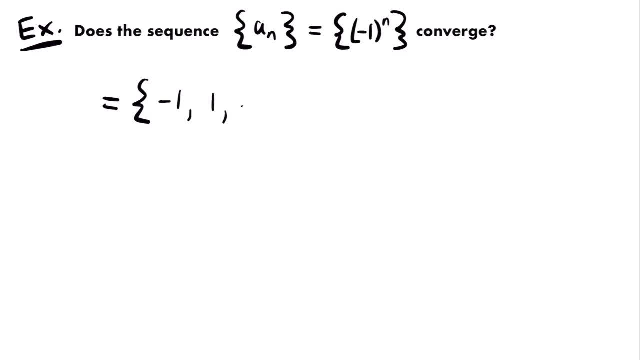 So if we write out the first few terms, we have negative 1, 1,, negative 1, 1, and so on. All right, so those are the first four terms. We're just oscillating between those two values. 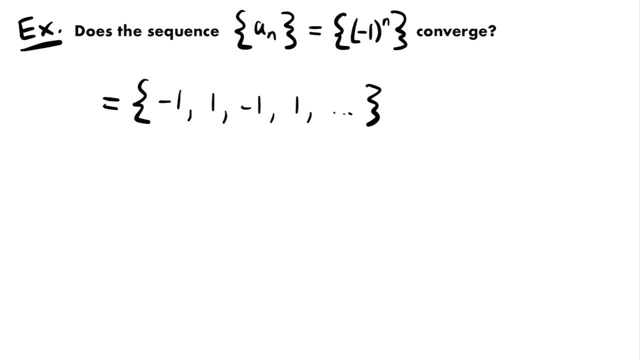 And so can you determine, by looking at these values, that this sequence is either increasing or decreasing. Well, since our terms are oscillating between two specific values, it's not increasing or decreasing. Each subsequent term is not greater than the previous term, and so it's not increasing. 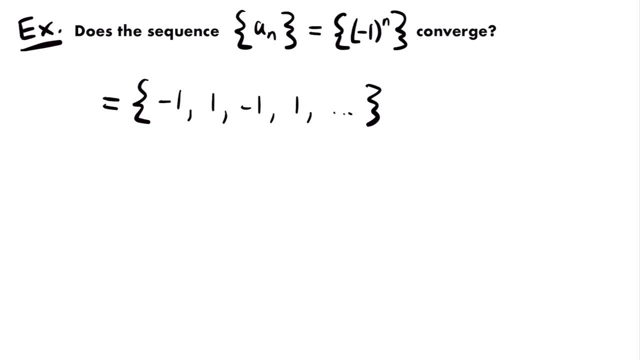 And each subsequent term is not less than the previous term, and so it's not decreasing. And so, since this sequence is oscillating, we know that it is not monotonic. all right, So we can stop right there. We could just say that we don't know if this sequence converges because it's not monotonic. 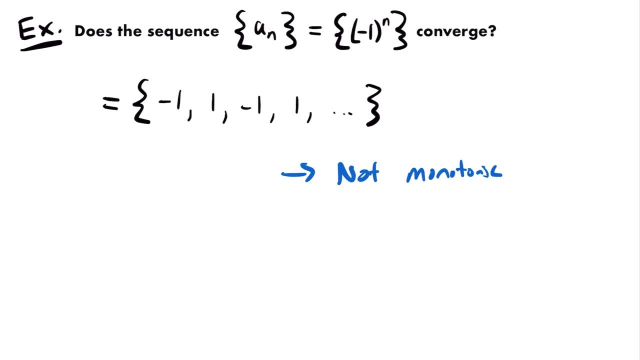 But let's also see if it's bounded before we make our final conclusion. And so let's graph our terms here. Remember that the horizontal axis is the values of n, and then our terms are the vertical axis, And so we're just going to look at the first four terms here. 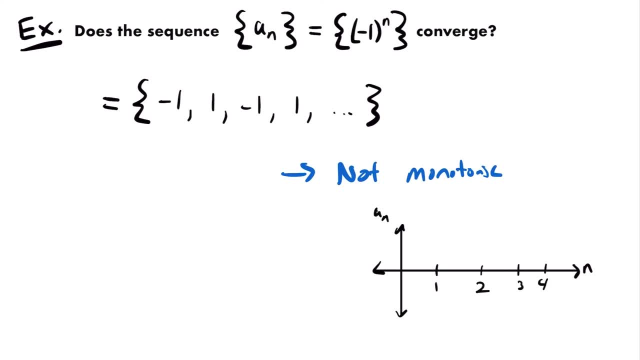 So we have n equals 1,, 2,, 3, and 4.. And the only values that they are going to be are either positive 1 or negative 1.. And so if I graph each term, when n is equal to 1, the term is negative 1.. 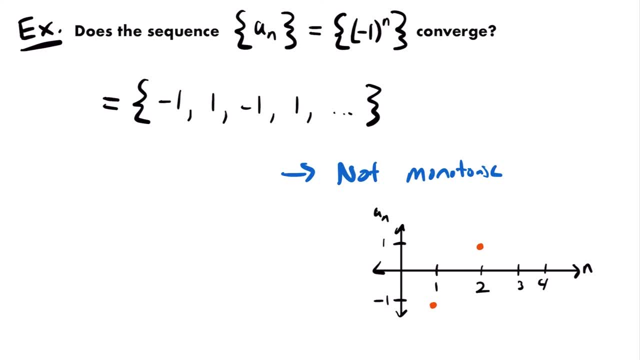 When n equals 2,, the term is positive 1.. When n equals 3,, we're back to negative 1. And when n equals 4, we're back to positive 1. And so our sequence here is oscillating between those two values, as we know. 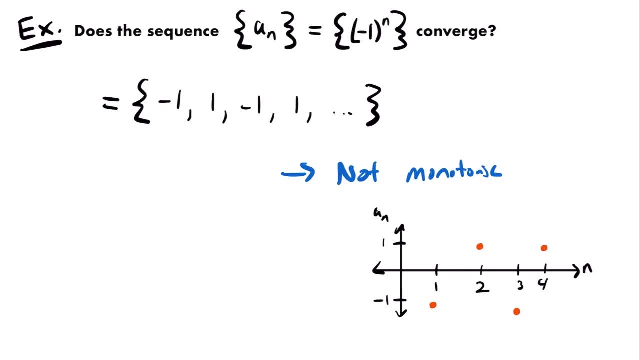 But is it bounded above and below by some value? Well, since we know that the terms are either going to be negative 1 or 1, we know that the terms will never be greater than 1.. And they're also never going to be less than 1.. 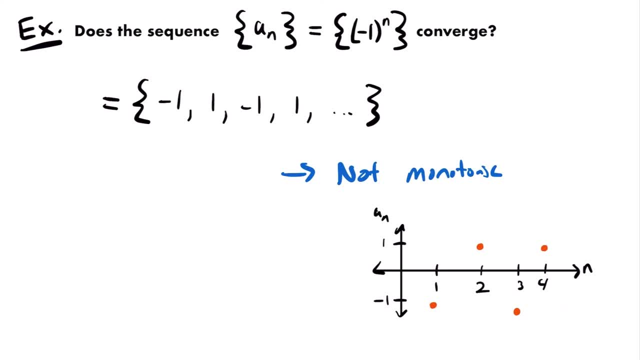 So we're just going to look at the first two terms here. The first two terms are going to be less than negative 1.. And so this sequence actually is bounded, because it's going to be bounded above by m, where m is equal to 1.. 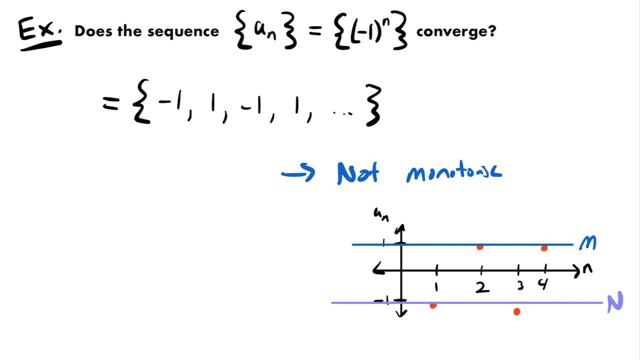 And it's going to be bounded below by n, where n is equal to negative 1.. Now that dot right there is a little bit lower than it should be, And so if I fix that real quick, it should be right at negative 1.. 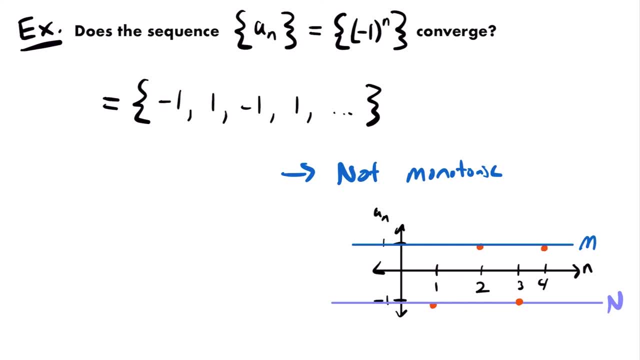 It shouldn't be below that line, But anyway, you get the idea that this sequence is bounded above by m, where m is equal to 1, and bounded below by n, where n is equal to 2.. And so our sequence: a sub n is less than or equal to 1, but greater than or equal to. 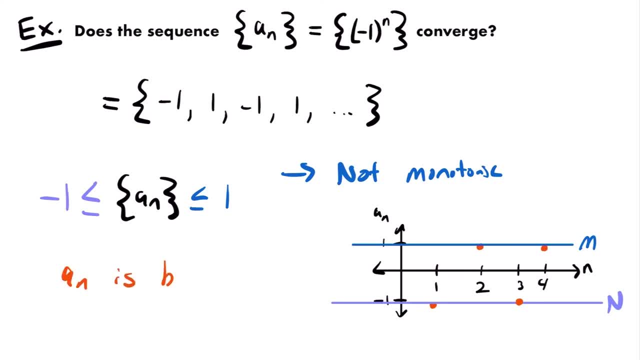 negative: 1.. Alright, so a sub n is bounded, but it's not monotonic, and so we cannot conclude that it converges. Now be careful here. Just because it doesn't meet both requirements doesn't mean that it does diverge. 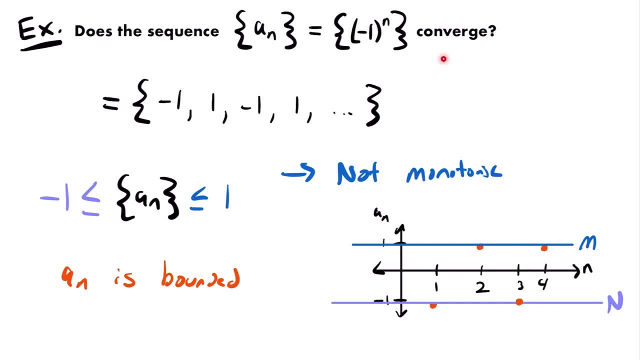 A lot of people will assume that well, since I couldn't prove that it converges, then it must diverge, And that would be an incorrect way to go about things. Just because we couldn't prove that it converges doesn't necessarily mean that it diverges. 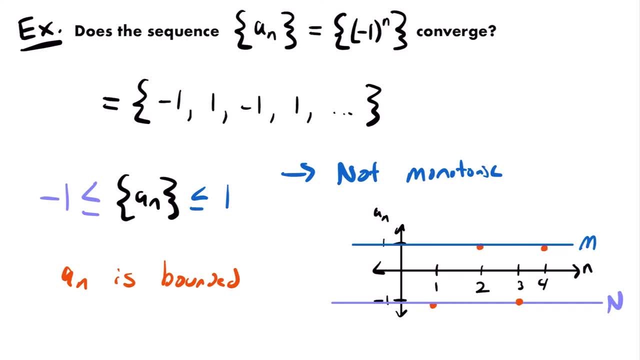 All we can say is that this test is inconclusive. We're not able to decide if this converges purely based on if it's monotonic and bounded, Alright. but now this specific sequence does diverge because it's oscillating between two values.